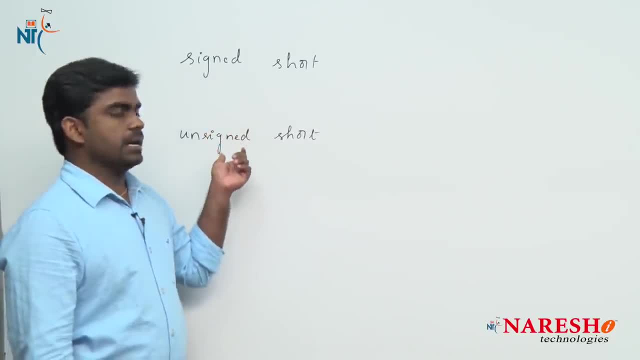 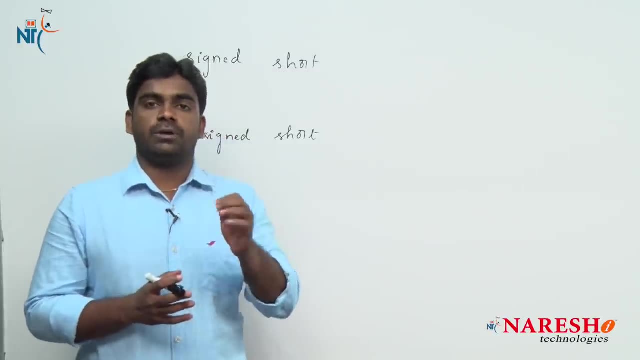 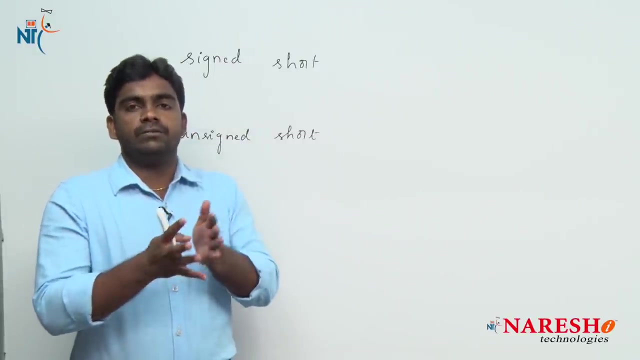 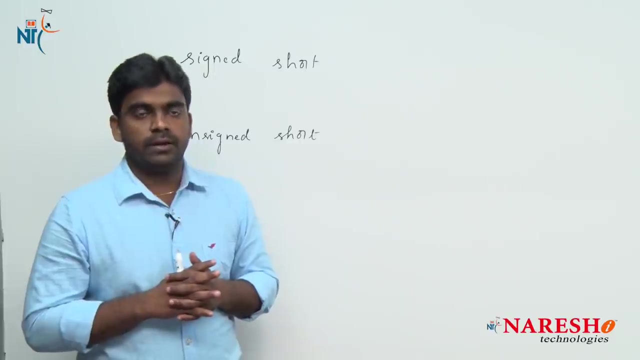 unsigned. So what is a signed data type and what is a unsigned data type? means: Using signed, we can store only a positive value, But using signed data type, a positive value and negative value also we can store. Using unsigned We can store only positive value. right, and what is the size of shot? either, it is a signed. 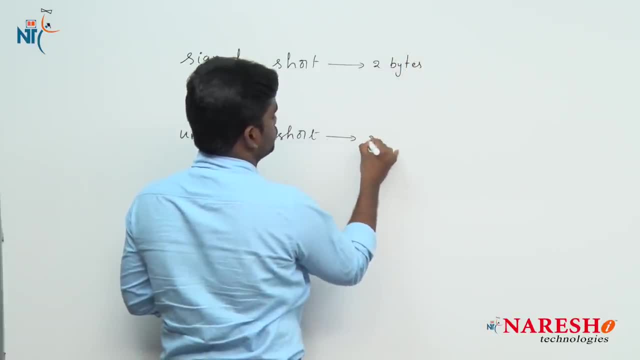 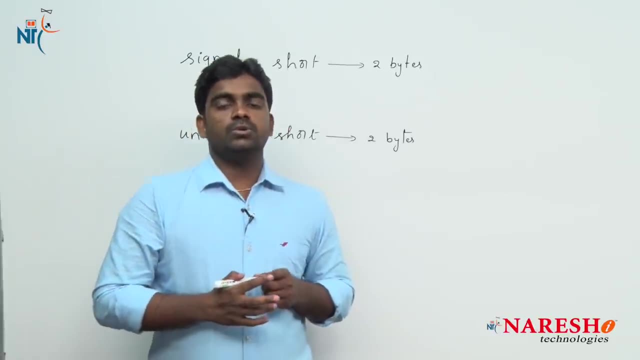 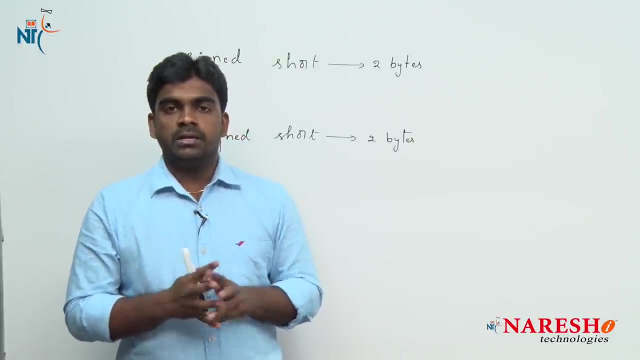 shot or it is unsigned shot. it occupies 2 bytes memory. How many bytes? It occupies 2 bytes memory. So, using 2 bytes memory. so what is the minimum value we can store and what is the maximum value we can store? Just look at the memory allocation process. 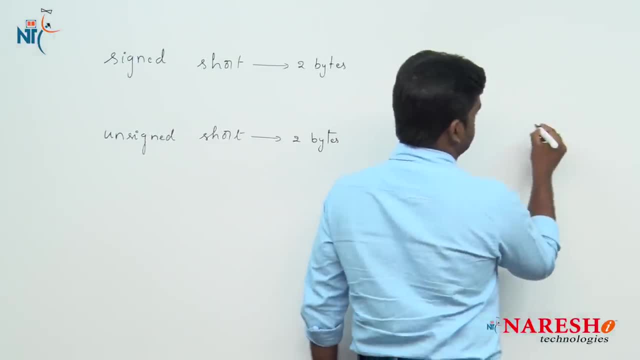 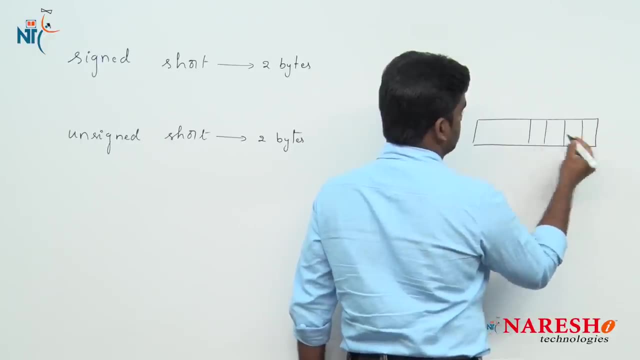 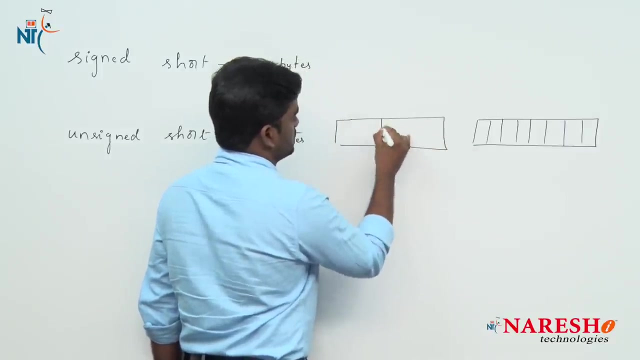 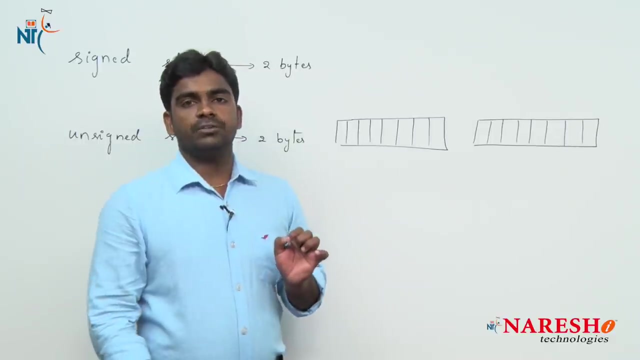 Here, suppose, 2 bytes memory I am taking. this is the first byte, this is the first byte I am taking first byte and this is a second byte is a second byte. So, using 2 bytes memory, what is the minimum value we can store right? 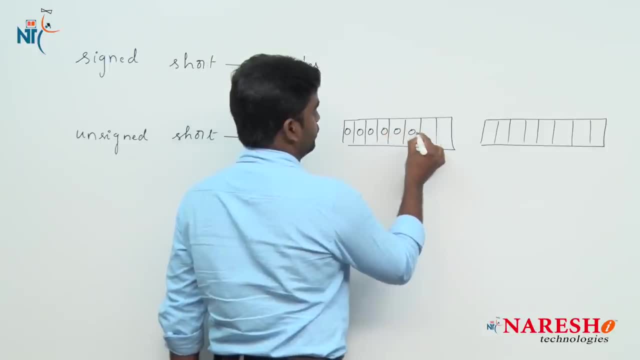 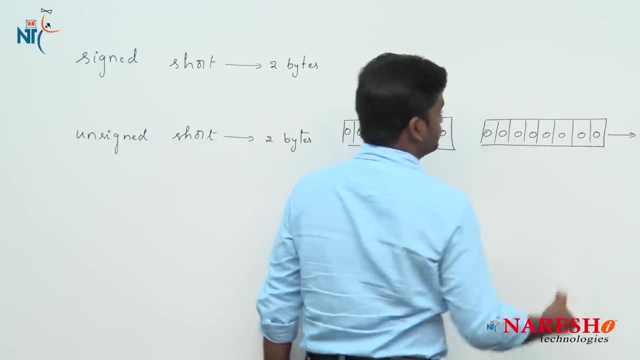 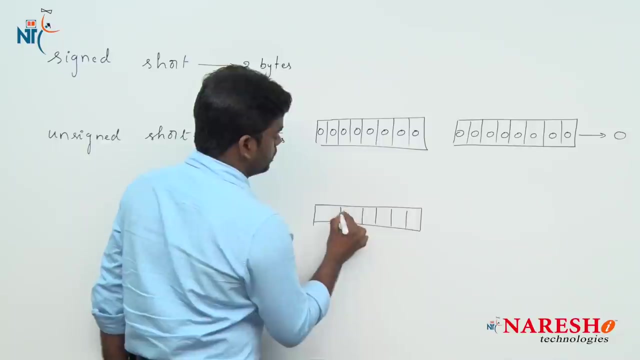 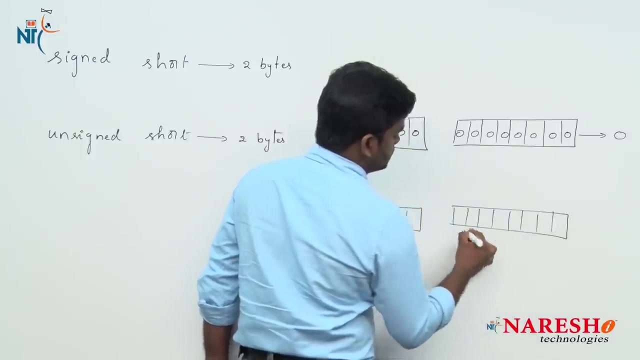 So the data will be stored in the form of binary values. So if you place all are zeros, all are zeros, the minimum value is a 0 and the maximum value, what is the maximum value we can store using 2 bytes memory? using 2 bytes memory, is we? 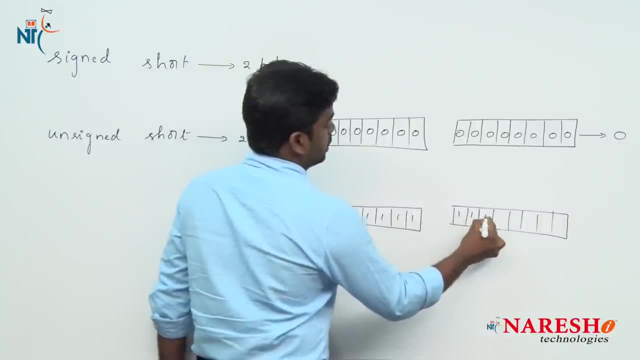 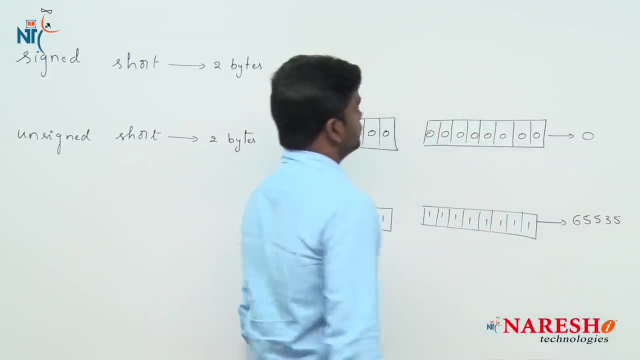 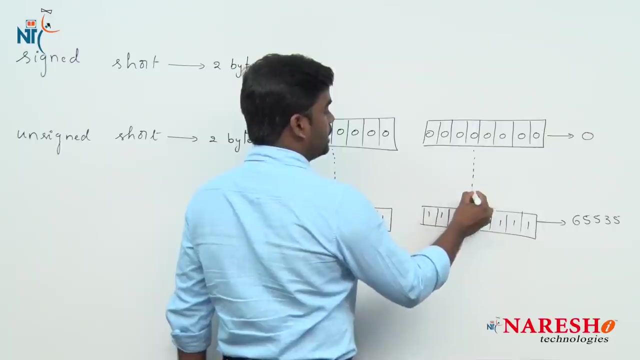 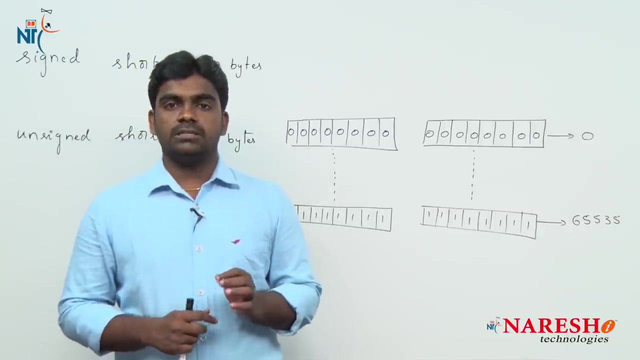 need to place all ones, all 1. 1. 1. 1. 65535.. So, using 2 bytes memory, a minimum value, a minimum integer value we can store is a 0 and the maximum integer value we can store is a 65535, right? So here it is a simply. 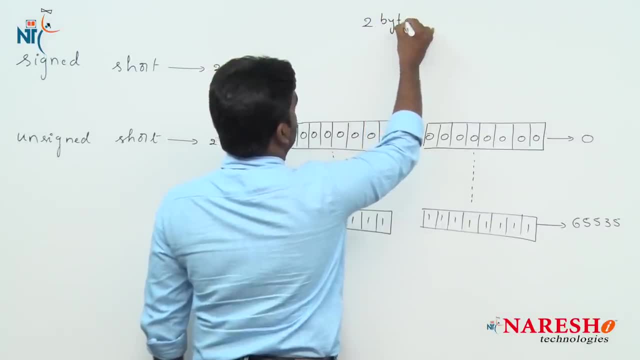 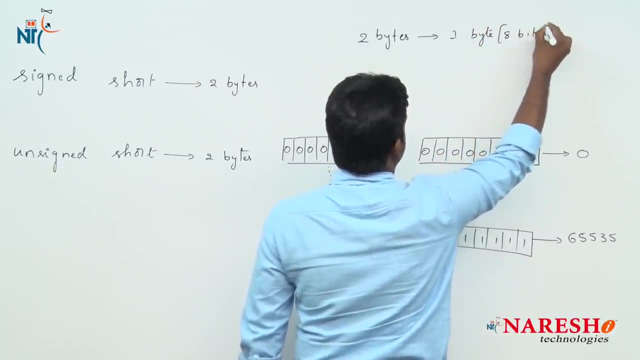 how can we understand? means is a 2 bytes? means 1 byte is equals to 8 bit. 1 byte is equals to 8 bits, So 2 bytes is nothing but a 16 bit. So we have to calculate 2 power 16 value. 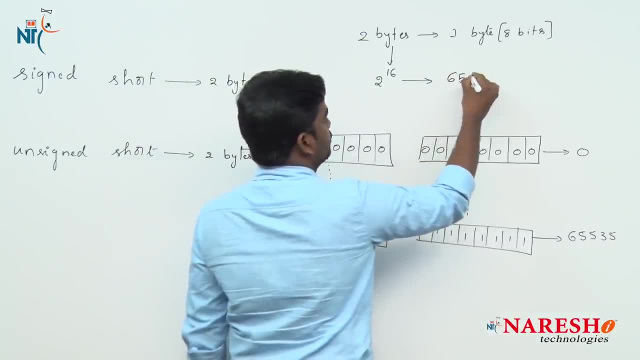 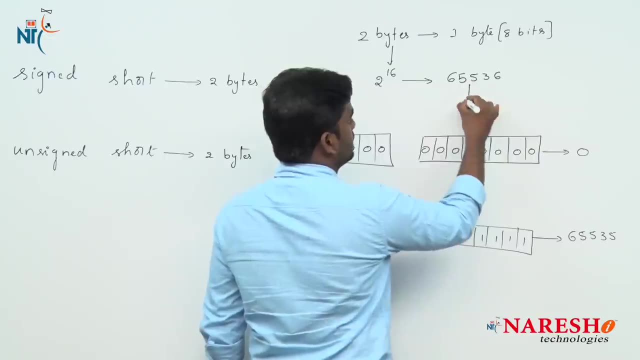 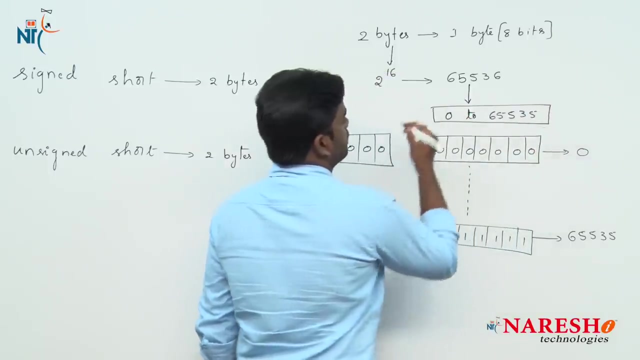 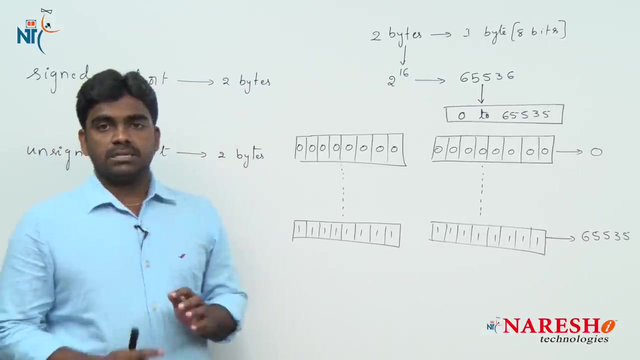 2, power 16 value is a 65536, but here it is a storing value starts with a 0. So here it is a 0 to 65536.. So what is that unsigned data type? and what is a signed data type means unsigned always. 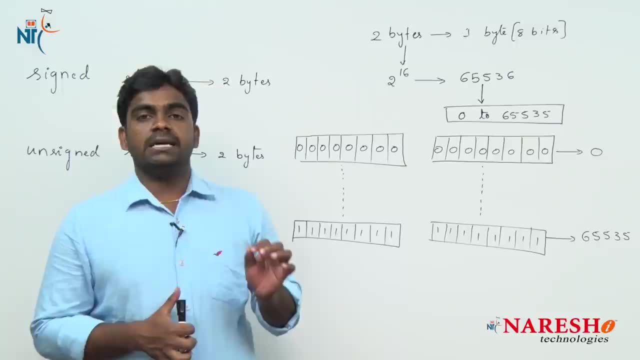 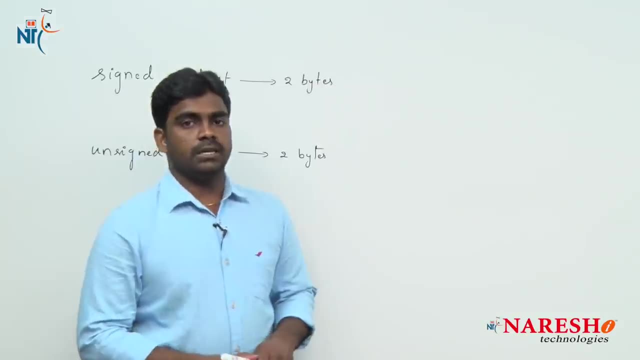 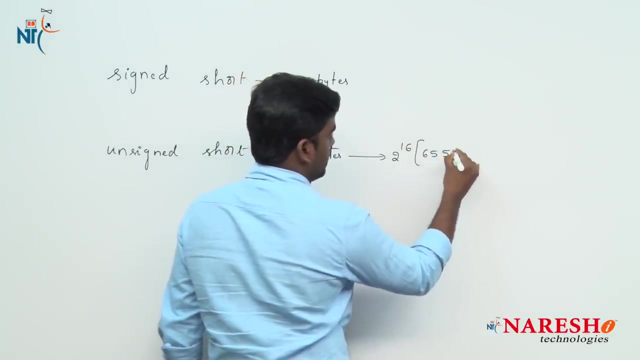 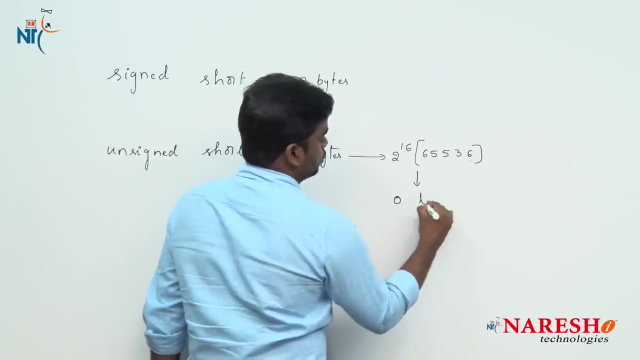 stores a positive value. So the range of unsigned data type is 0 to 65535. here it is 2 bytes. So we need to find out the value 2 power 16, the value is a 65536.. So 65536, and here it is a range 0 to 65535. this is a minimum value we can store and this 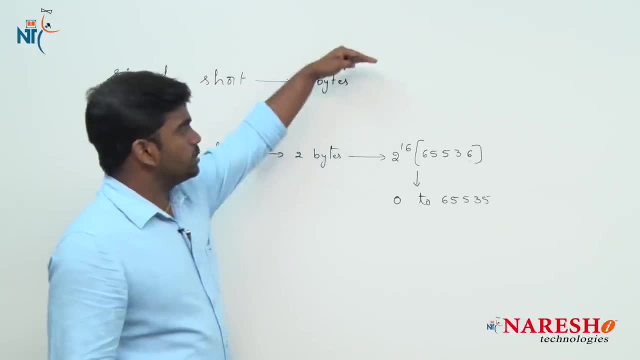 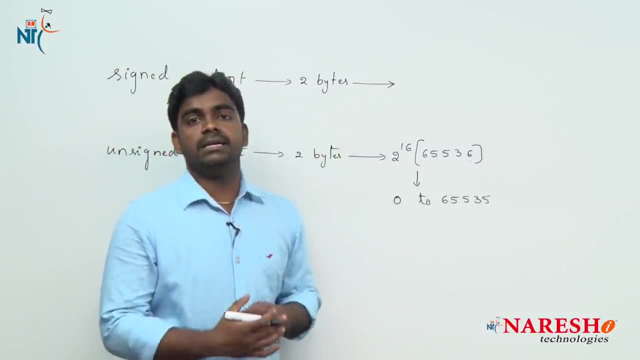 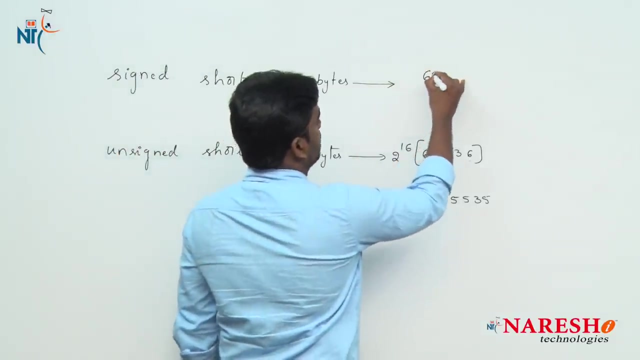 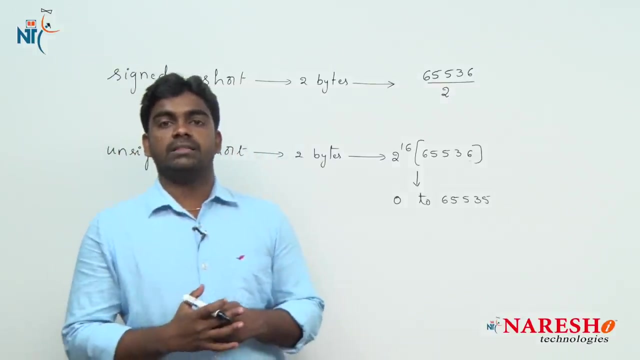 is a maximum value we can store. and next one- come to this point here- it is using 2 bytes, using 2 bytes signed data type. Now, what is the minimum value and what is the maximum value? So up here it is 65536 by 2. just divide the value 65536 by 2 if you divide. So what? 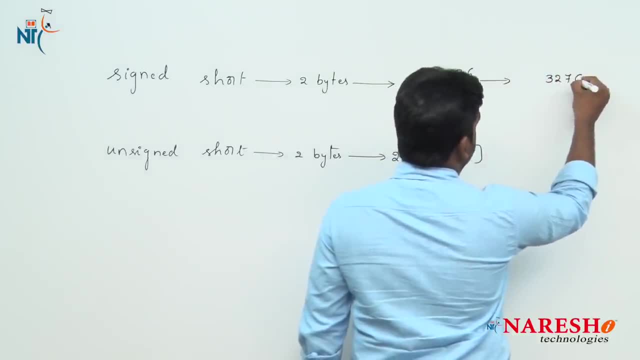 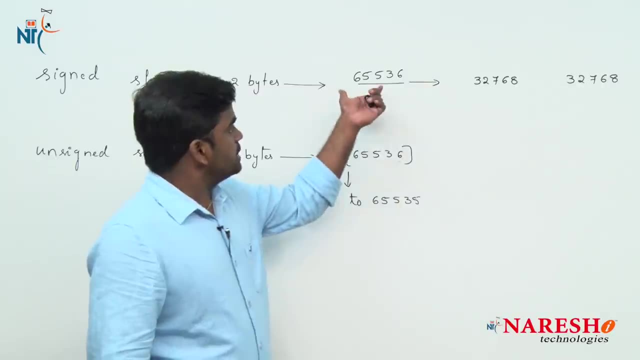 is the value. This is 3, 2,, 7,, 6,, 8, and here it is 3, 2,, 7,, 6, 8.. This is half half of 65536.. So negative values always starts with a minus. 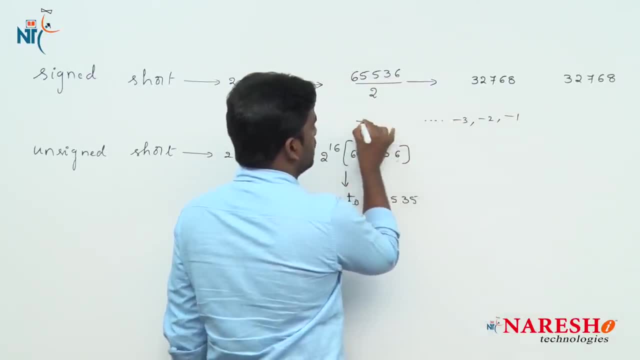 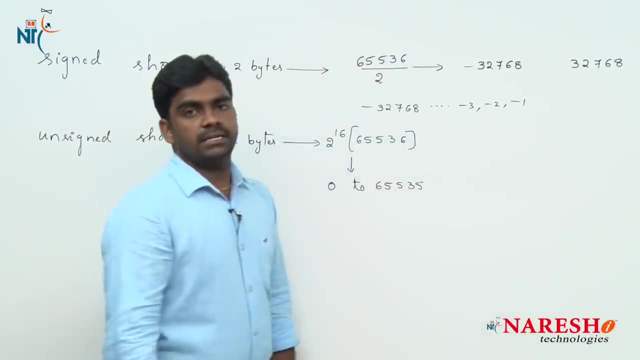 1, minus 2, minus 3,, minus 4, plus 5, minus 6, minus 8, three times minus 4 and half minus 2, minus 3, and so on. minus 3,, 2,, 7,, 6, 8 is ok. So negative values up to minus 3,, 2,, 7,, 6,, 8. 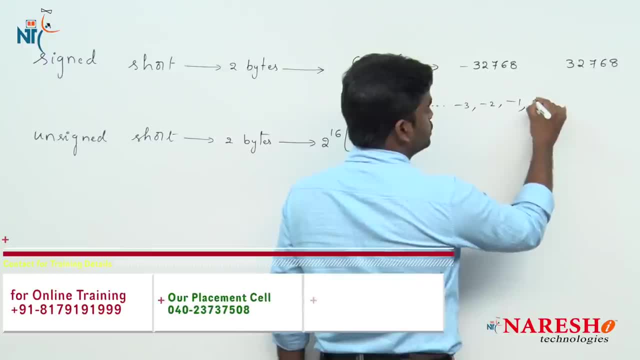 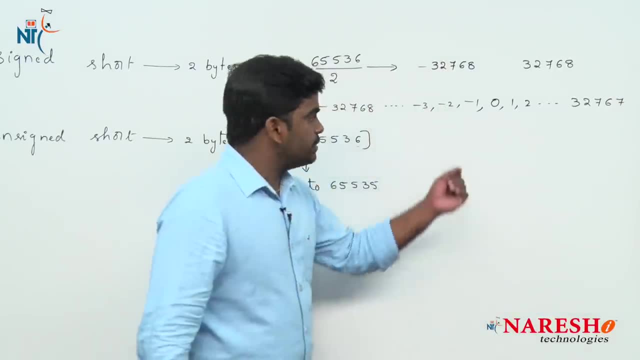 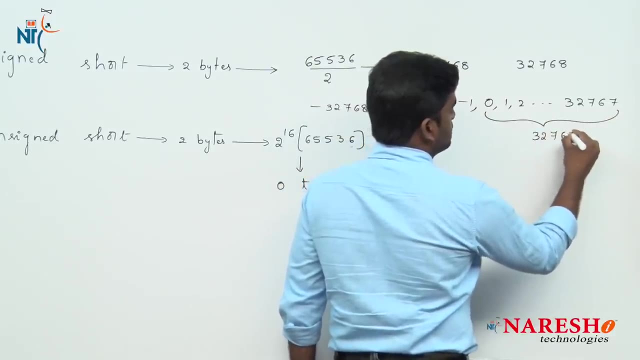 but here it is a positive values starts with a 0,, 1,, 2, and so on up to 3,, 2,, 7,, 6,, 7. only, sir, why? because we have to include 0 also, right, 0 plus 3,, 2,, 7,, 6, 7.. So total: 3, 2,, 7,, 6, 8 values. 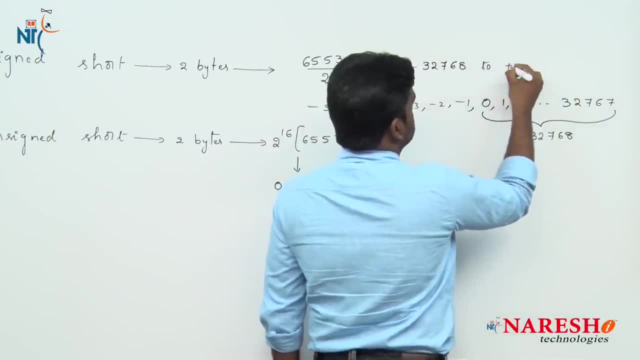 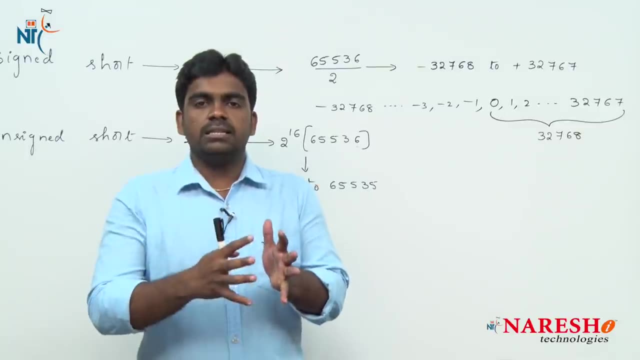 So range minus 3,, 2,, 7,, 6,, 8, 2 plus 3, 2,, 7,, 6, 7 plus 3, 2,, 7,, 6,, 7.. So these are the limits. 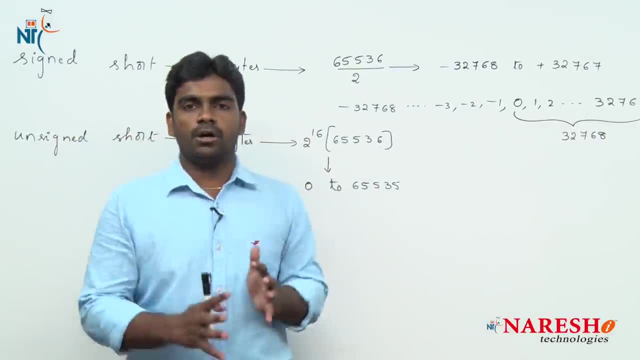 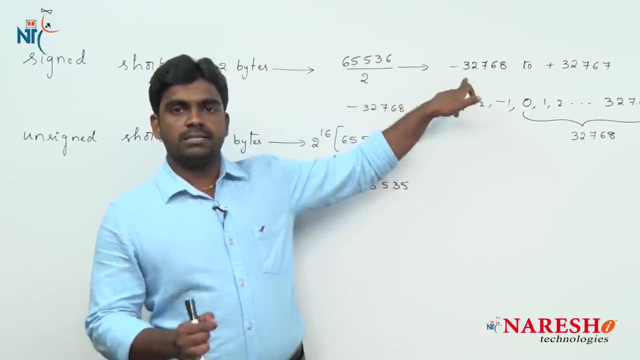 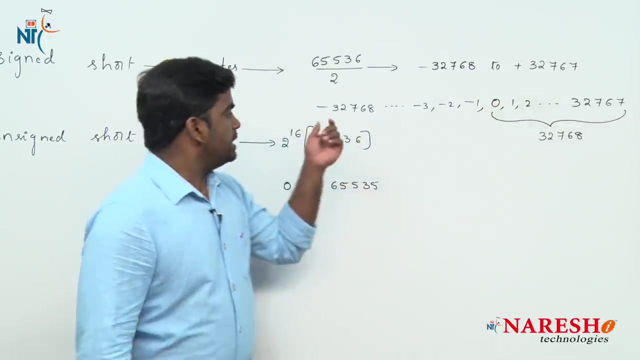 of short data type, either signed data type or unsigned data type. using signed data type. So what is the minimum value we can store is a minus 3,, 2,, 7,, 6,, 8, and what is the maximum value we can store is a 3,, 2,, 7,, 6,, 7, and here it is using. 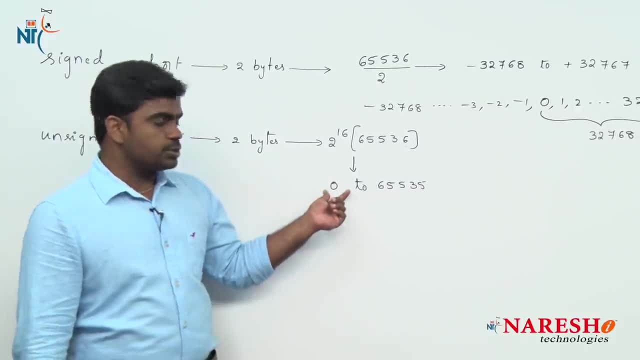 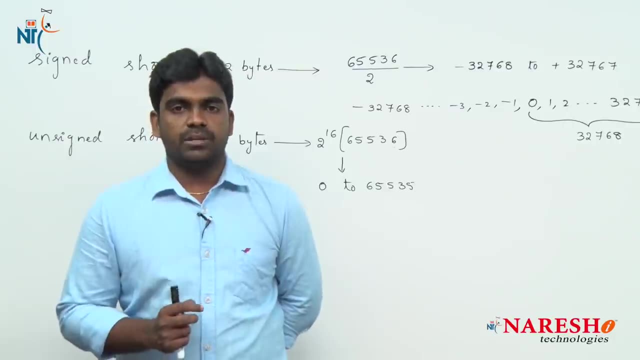 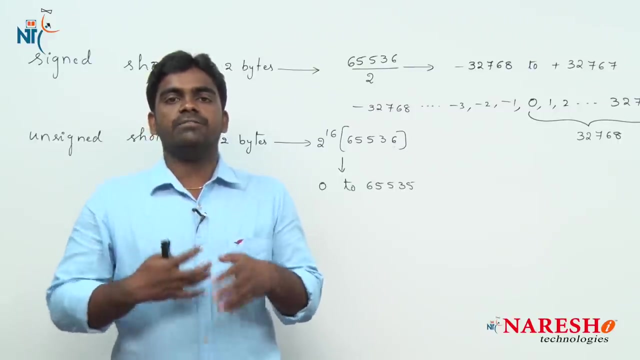 Unsigned short, the minimum value we can store is a 0 and the maximum value we can store is a 65,535.. So these are the limits of short data type, and next important discussion is in how many ways we can declare the short data type and the format specifiers of a short data type. 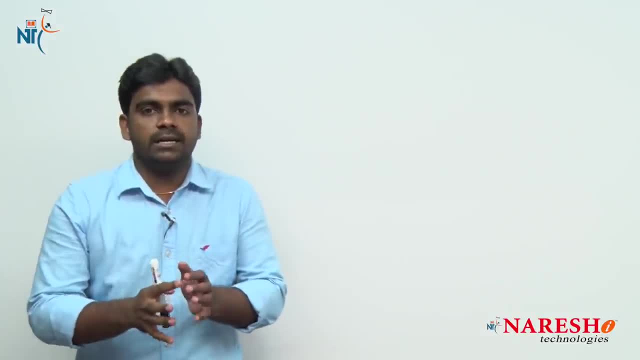 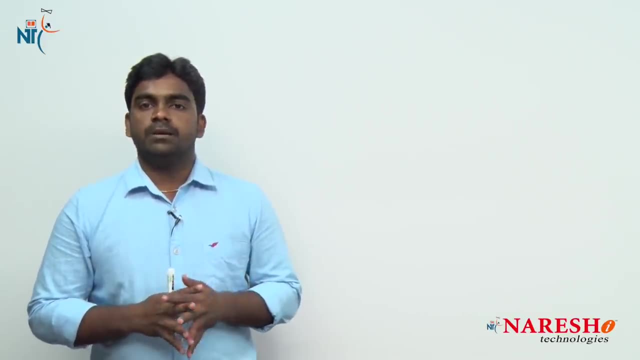 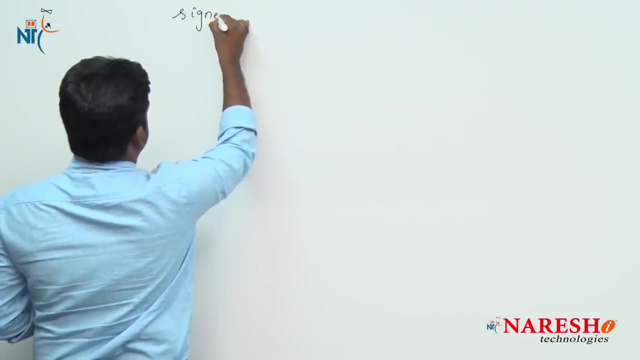 So what are these? C Now I just want to declare a signed data type variable in my program. signed data type variable in my program. How? Here suppose these are signed declarations, signed declarations and followed by unsigned declarations. also, we will see. 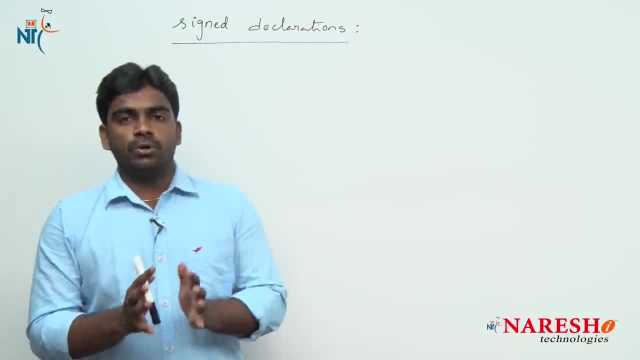 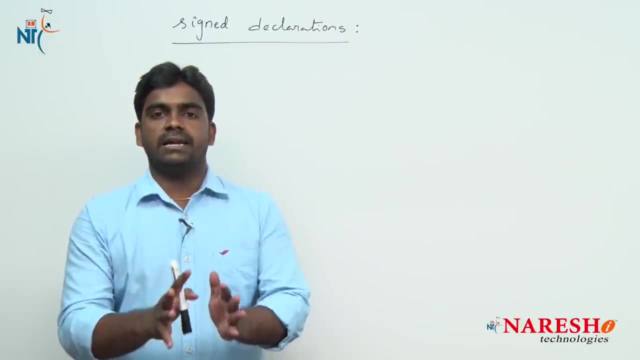 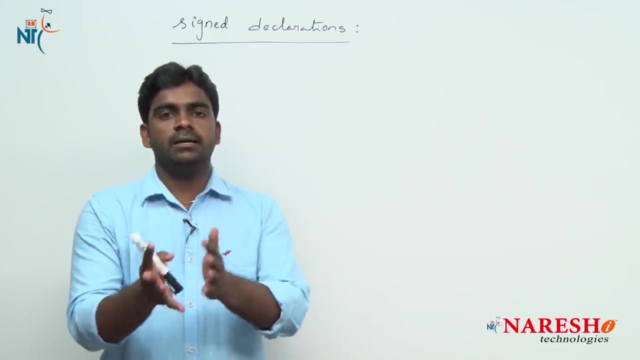 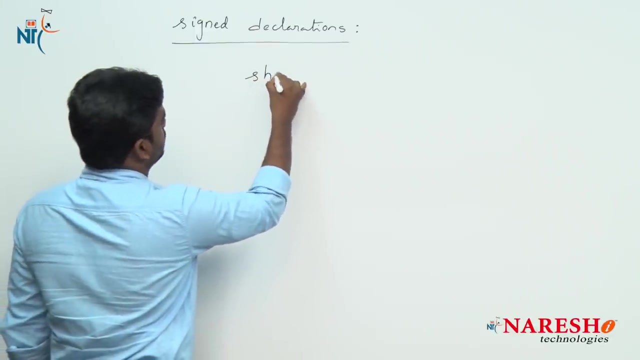 See in the declaration of variable, if you do not specify whether the variable is a signed variable or the unsigned variable, by default that is signed. by default That is signed. That means the variable accepts both the positive value and negative value. That is called sign data. Here it is simply: you can declare like this variable. short. 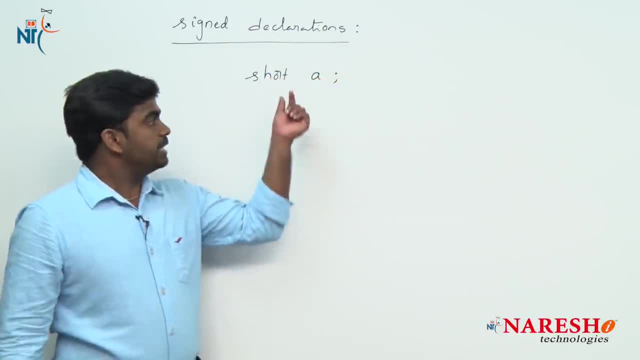 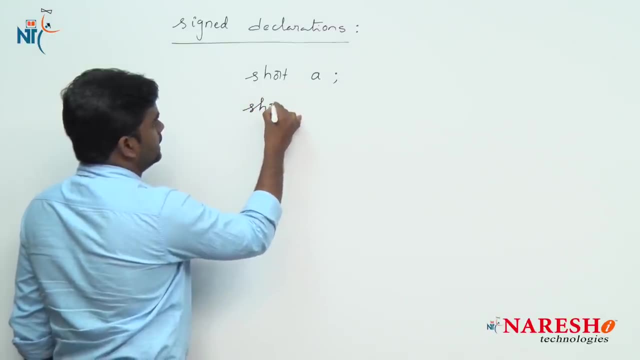 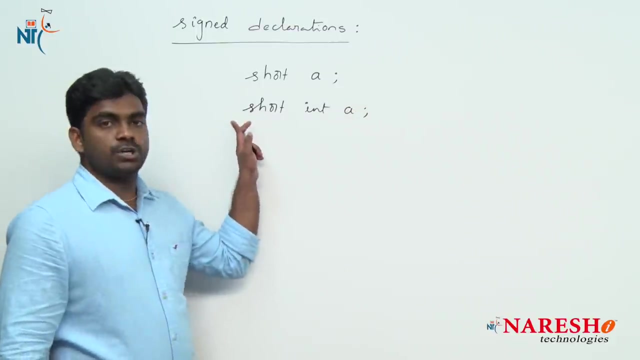 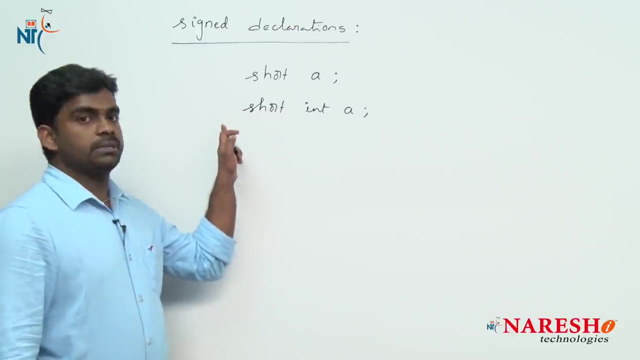 a. This is declaration of variable Variable a is of type short Write here. it is suppose if you want to write integer also, we can add short integer a. These two of type short type only. Sir, where is the signed or unsigned? I am not specifying, So by default these two variables are signed. 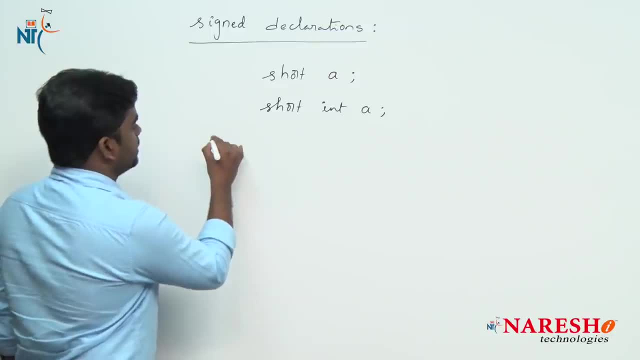 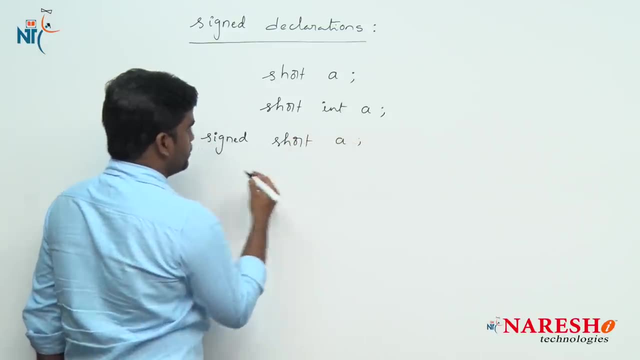 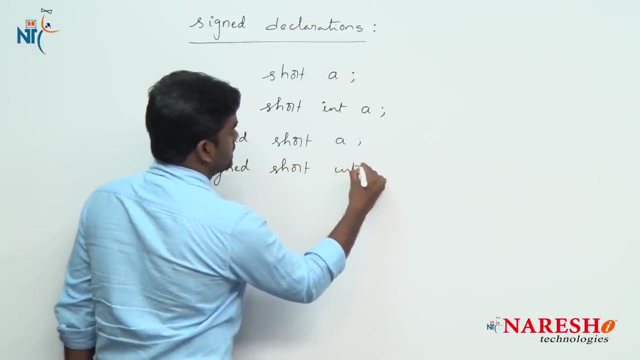 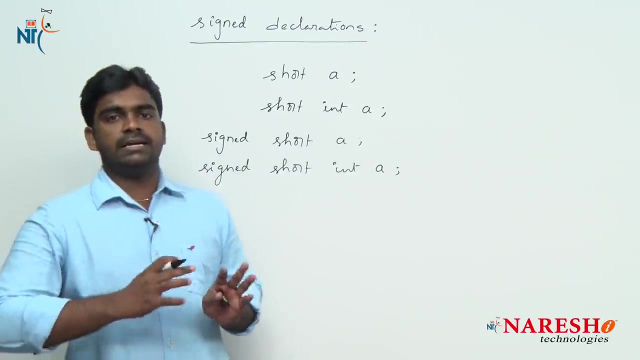 variables only. So here it is, Sir. can I write explicitly: Yes, you can. Signed short a, it is allowed and signed. complete declaration. last one signed short, integer a. In these many ways we can declare a signed variable into your C program, Sir. unsigned declarations. 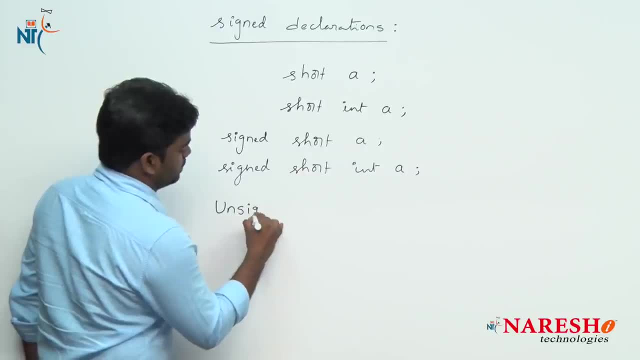 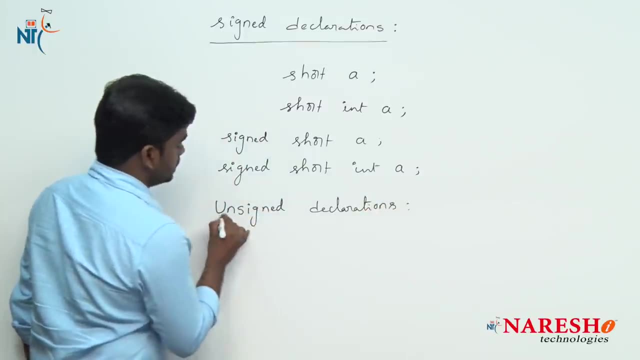 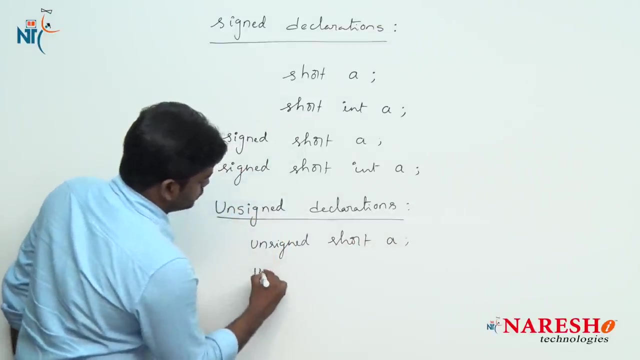 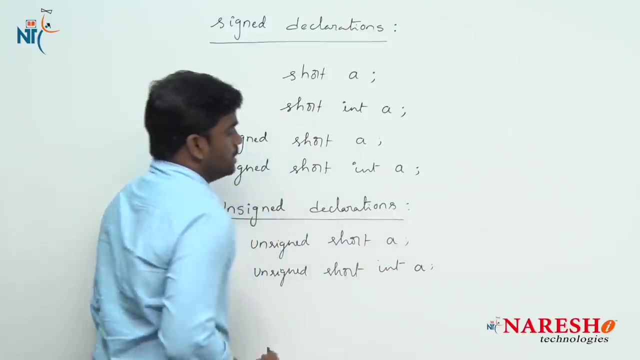 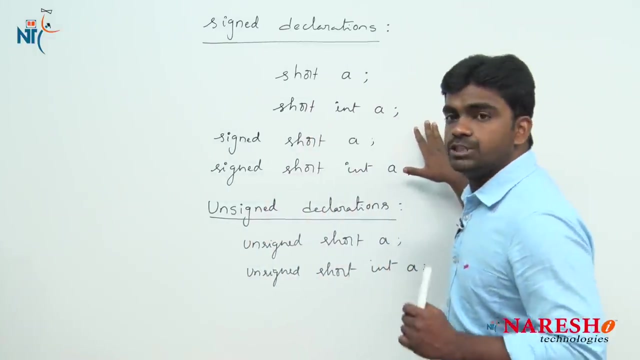 Here it is Unsigned declarations. we must specify explicitly These are unsigned declarations only two ways. First one is a unsigned short a and next one unsigned short integer a. So these are So total six declarations about a short data type. First four comes under signed short declarations and second 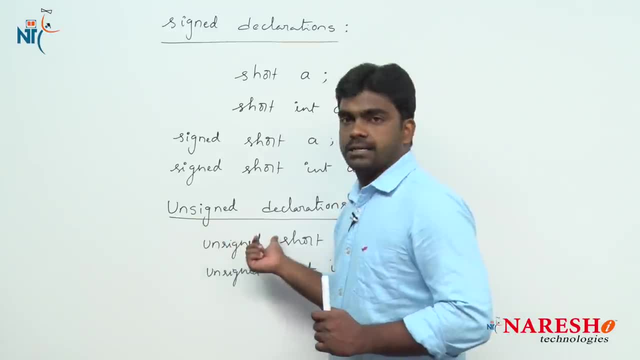 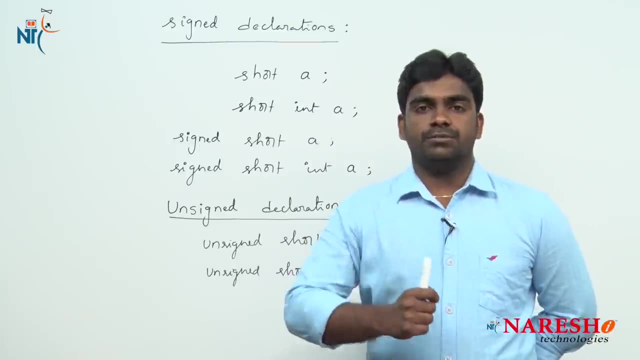 means what remaining two declarations comes under unsigned declarations, right, In these many ways we can declare. And the next important thing is format specifier. We can also call it as a format string in a C language. Sir, what is a format specifier and what is its importance? right, If you want? 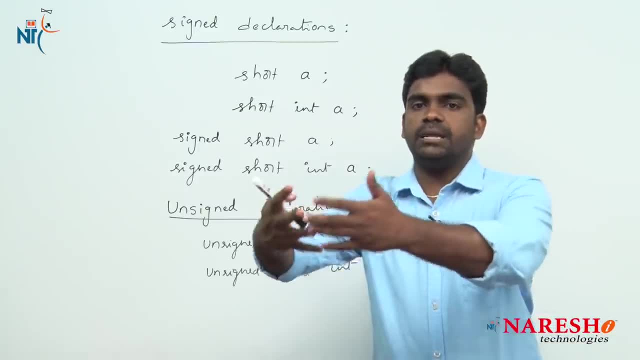 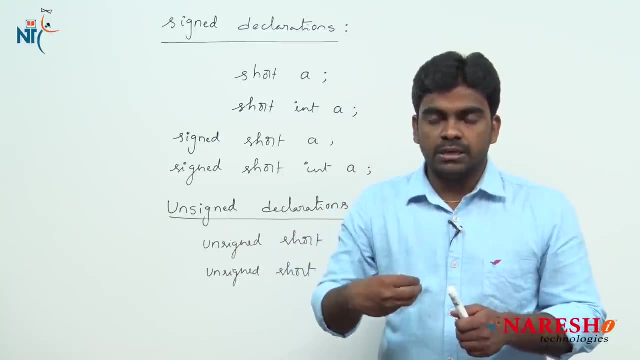 to read the information or if you want to display the information. formatting is very, very important, right, In which format you have to read the information, in which format you have to print the information that you have to specify to the C language. So this: 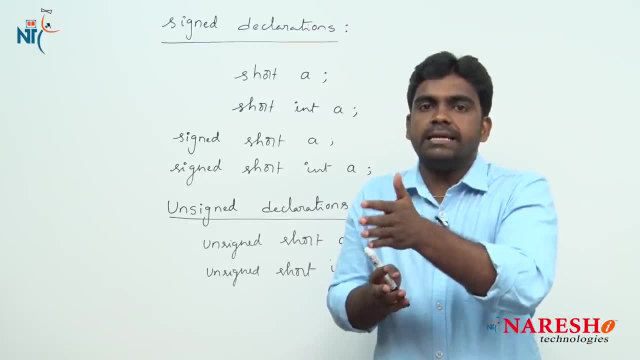 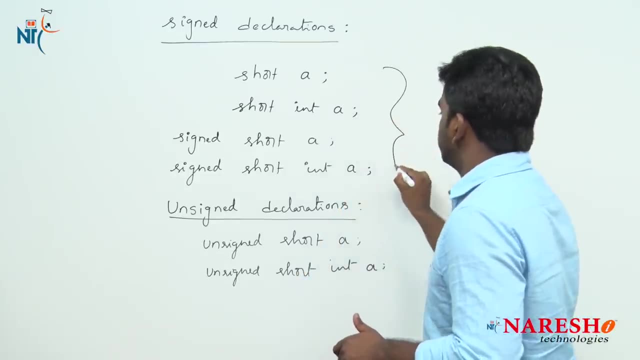 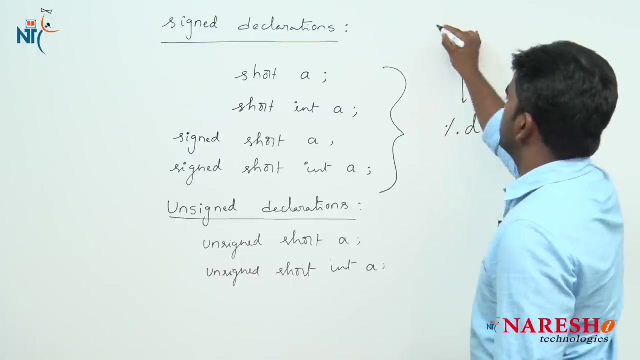 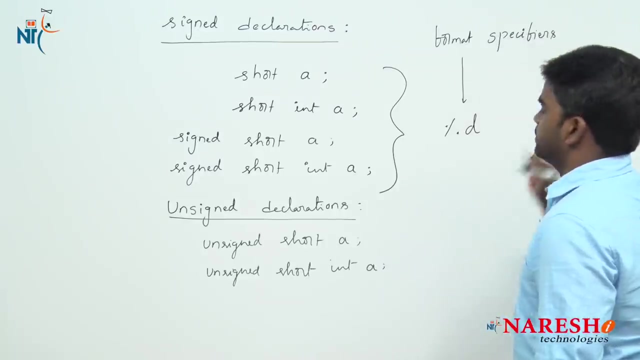 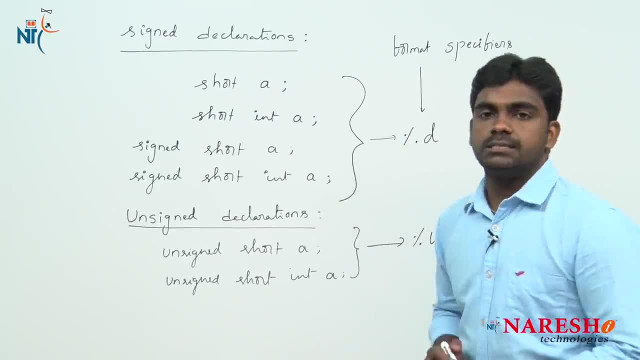 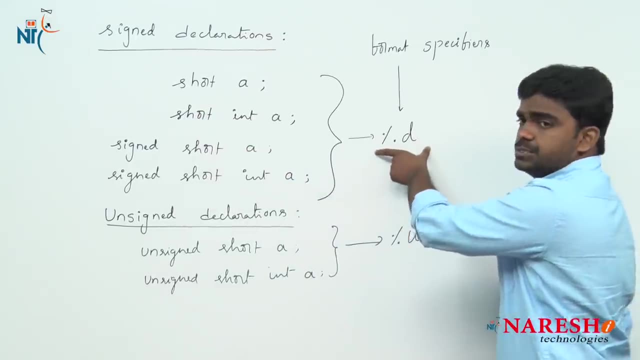 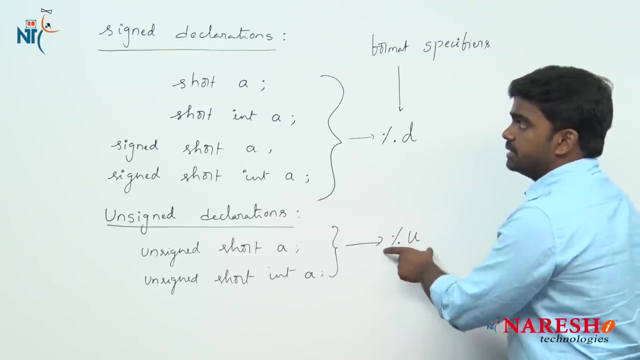 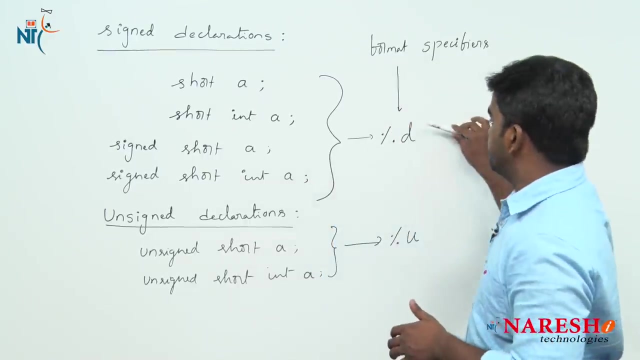 Format specifiers. The format specifier is a percentage u, Percentage u. These four signs declarations we are processing with the help of the specifier is percentage d and remaining two declarations, unsigned declarations we are specifying with a percentage u. these are signed and unsigned declarations of short time and here it is format specifiers we are. 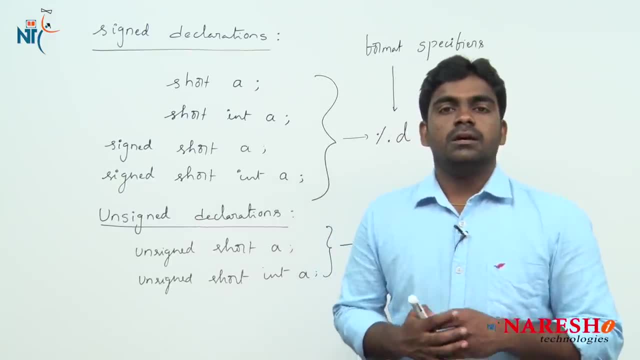 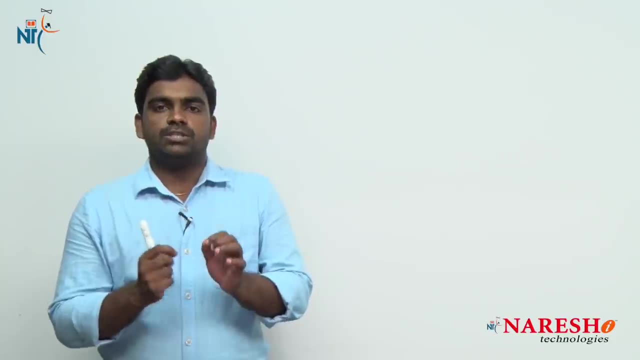 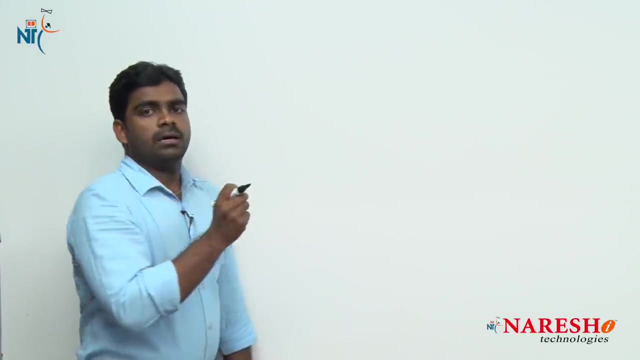 using Just an example. So based on these, so we will see right the programming on short data type. So now we will see. So some of the examples on a short data type, right see, For example, I just want to print a small value on the. 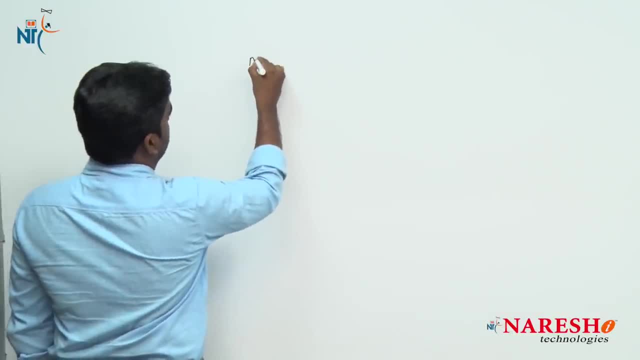 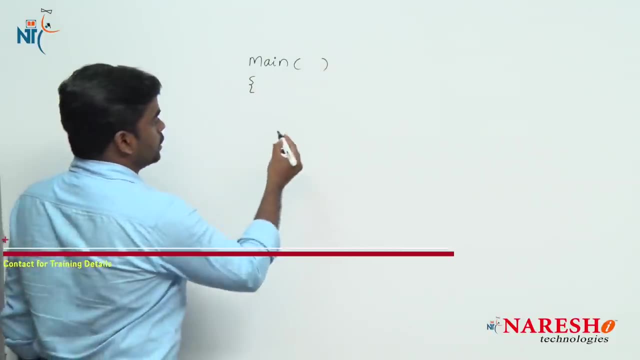 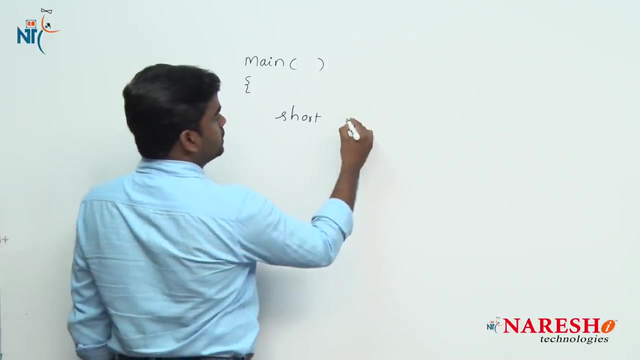 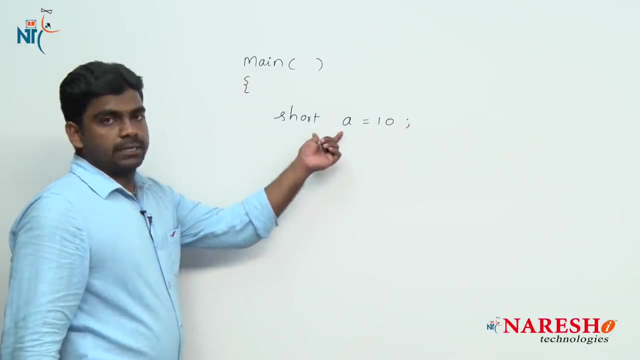 console. here it is. we are writing the program. execution starts from the main method. execution starts from the main method. and here it is. I am declaring one variable variable is a short variable. short, a equals to some value- 10. we are storing short, a equals to 10, and 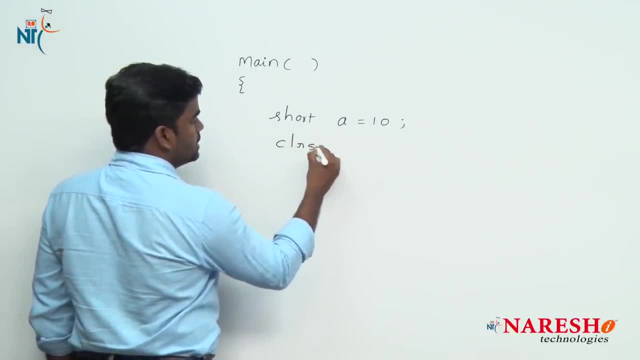 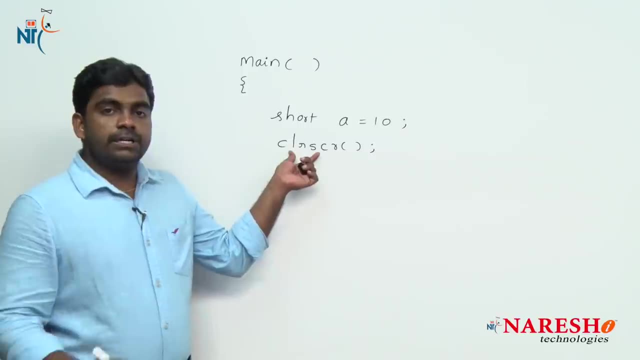 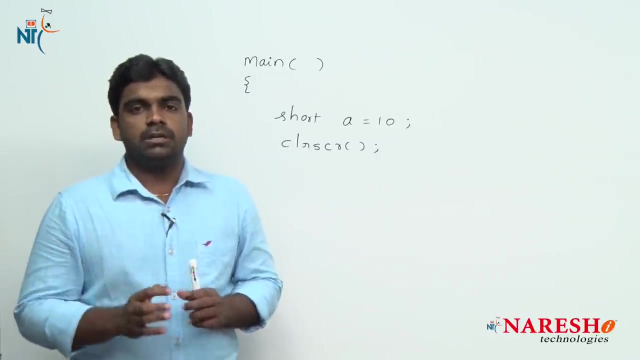 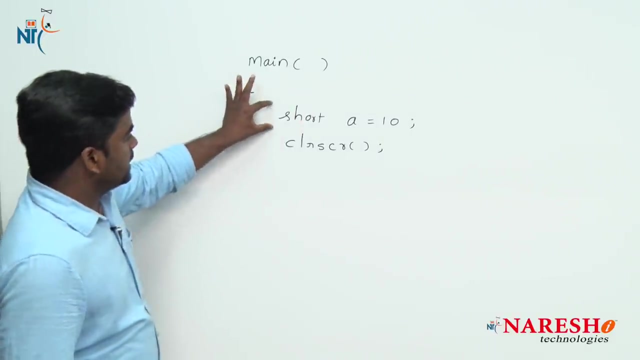 next, if you want to clear the screen: CLR, SCR, clear screen. remember clear screen always. we need to write After declaration of all the local variables. already we discussed in the local variables concept. all the local variables of a block you must place in the beginning statements. So after declaration. 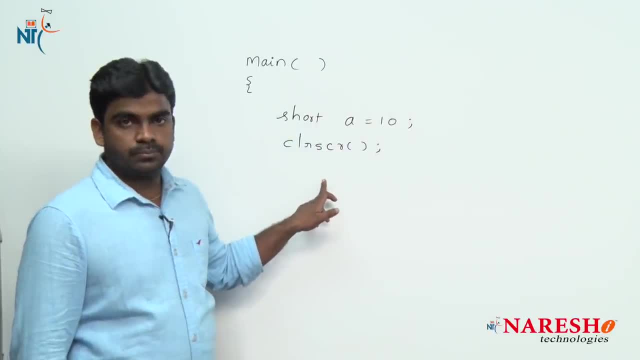 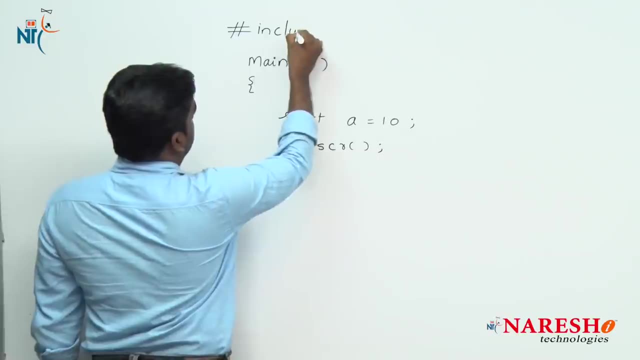 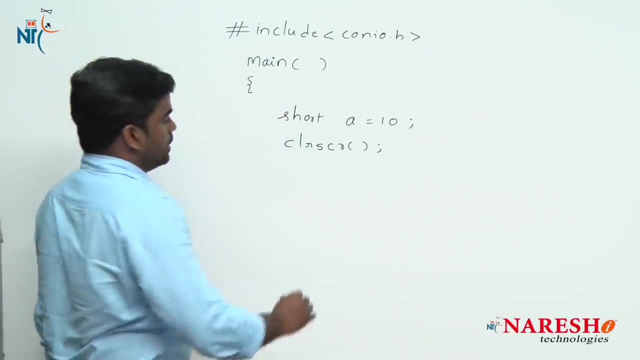 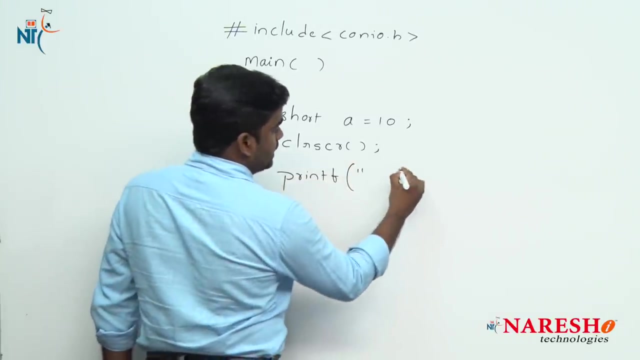 of all the variables, only you have to clear the screen. Next, clear screen function is available in a library. is a header file, c o n i o dot h. So I am including that. And next I want to print. So what is the function? printf function inside the double. 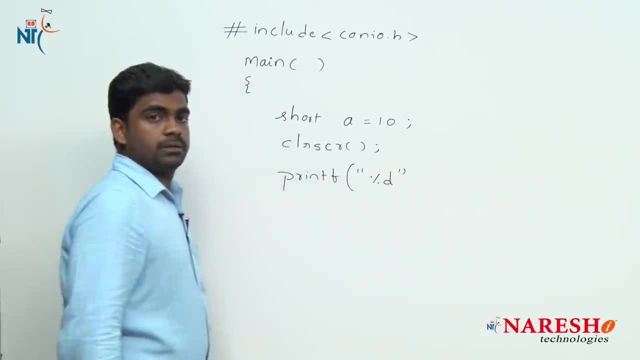 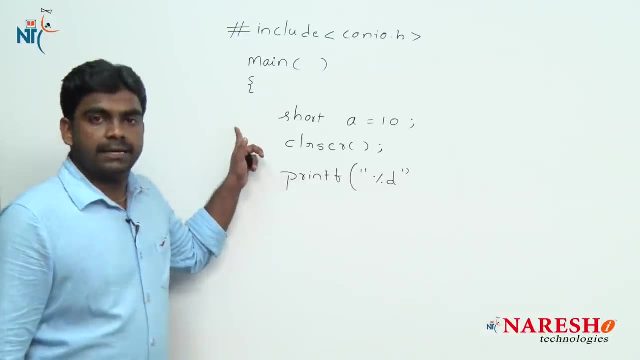 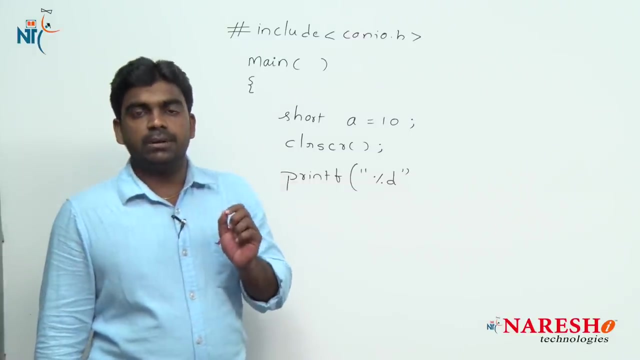 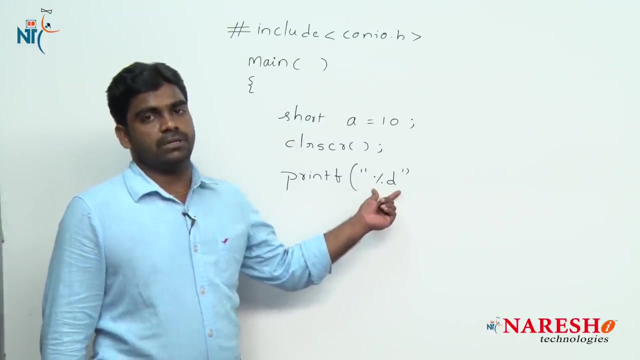 quotes. we have to write that format specifier. what format specifier? short format specifier? by default it is a signed. if you do not mention whether a variable is a signed variable or unsigned variable, by default it is a signed variable. So format specifier is a signed format specifier and here we are writing the variable that. 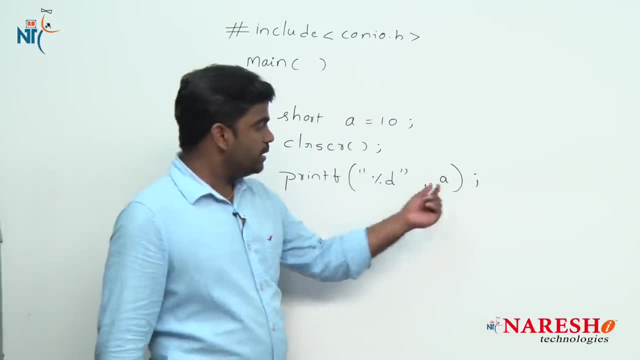 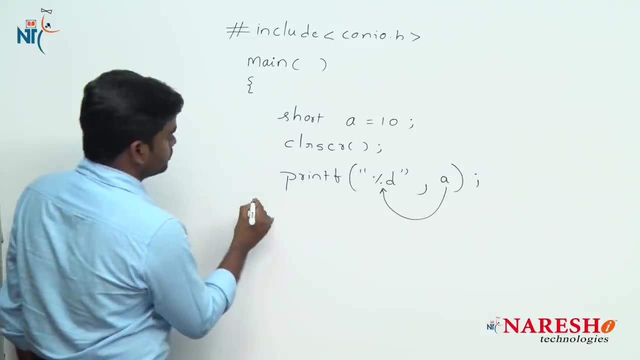 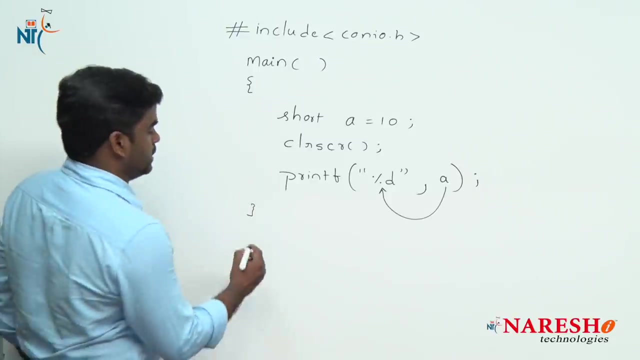 what you want to print. a is a variable. we just want to print So the value, variable value. it will print here in this place, in this place. So to this program. the output is right: 10 on the console. it will print the value 10. 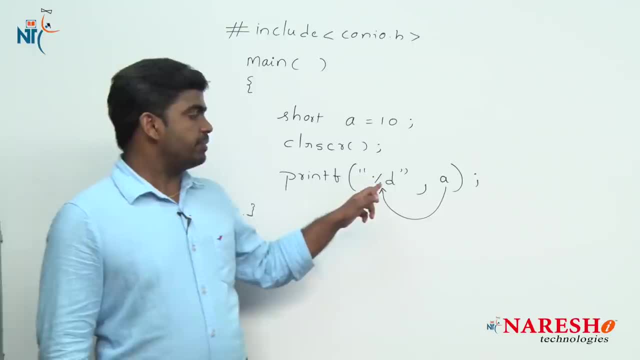 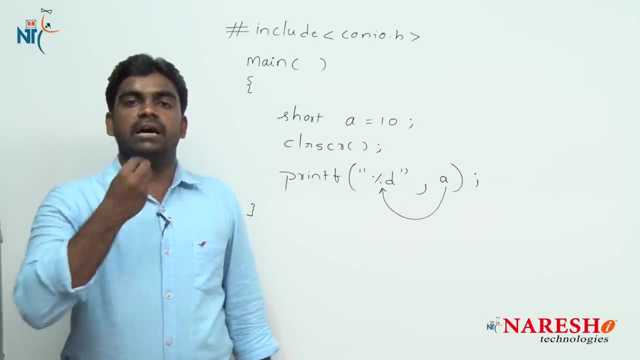 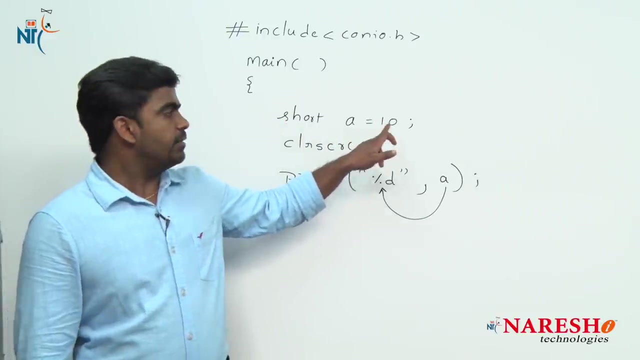 ok, So this is a simple program. here, format specifier is very, very important. with the help of format specifiers only, we are reading the elements and we are printing the elements Here. simply, I am declaring one short variable. right variable name is a, a with the value. 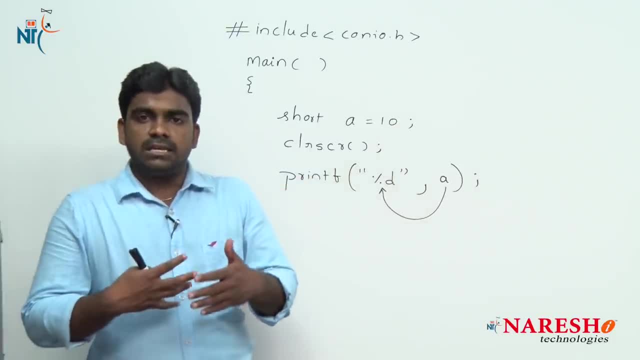 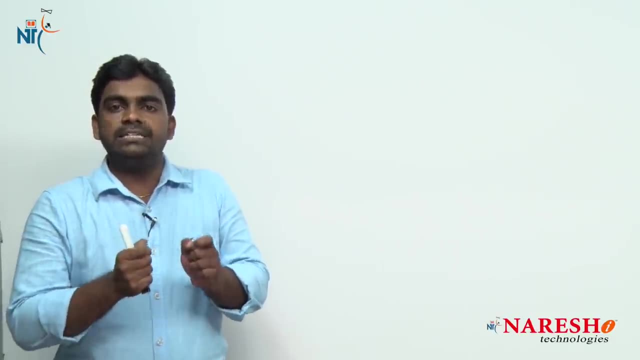 10.. So 10, it will print. So this is a simple program. Next we will see right some complex programs. ok, See. so first of all I am writing right the limits of a signed data type. I mean signed short data type in the form of circle. observe 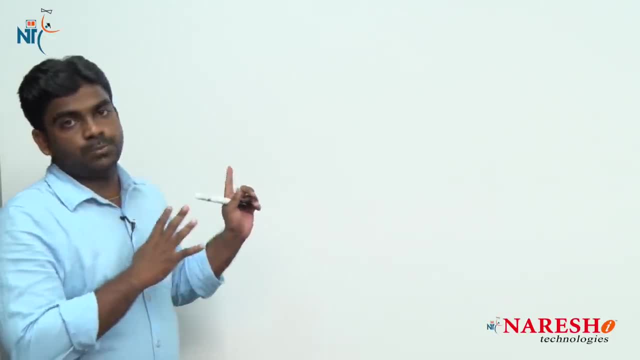 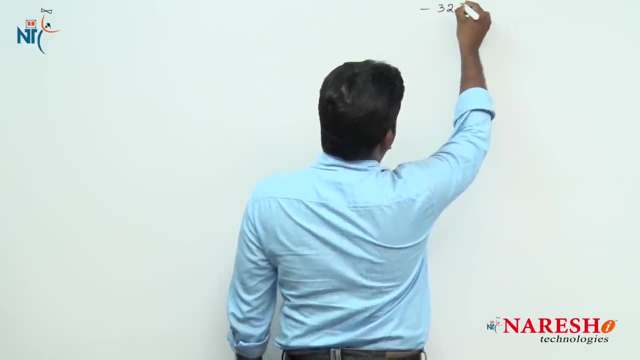 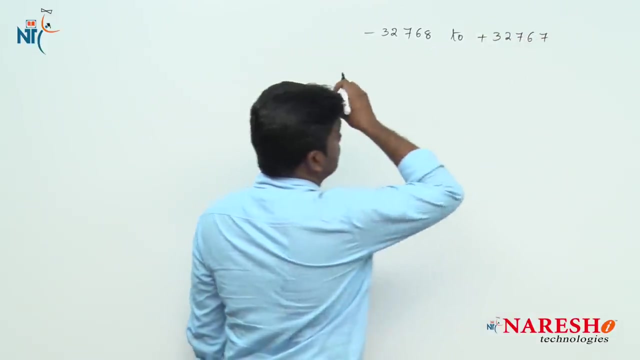 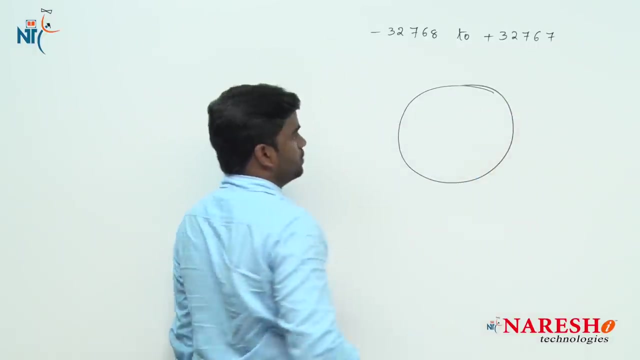 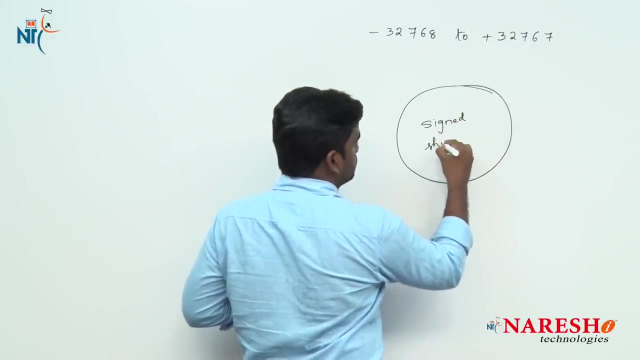 Because based on that circle, only now we are writing this program. observe, Here it is. this is a signed short circle. limits error: minus 327682 plus 32767. ok, These limits I am writing in the form of circle. observe, In the form of circle we are writing: this is signed short circle, signed short, that is. 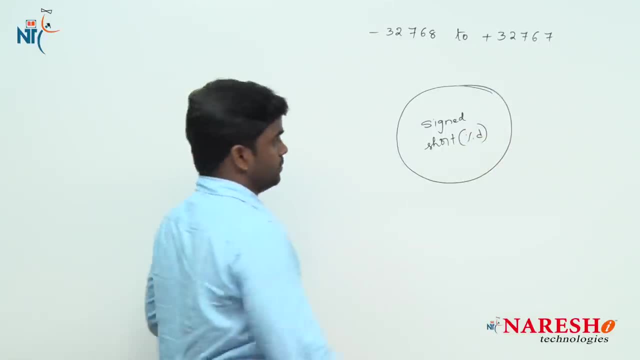 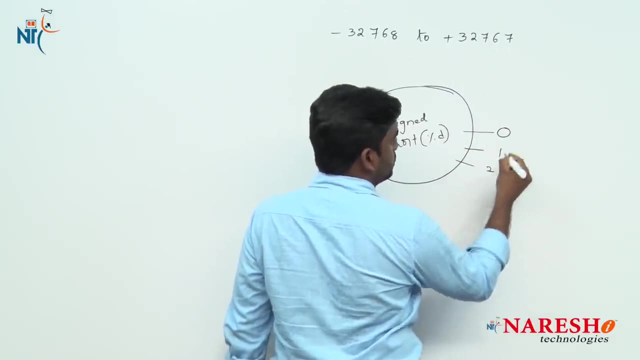 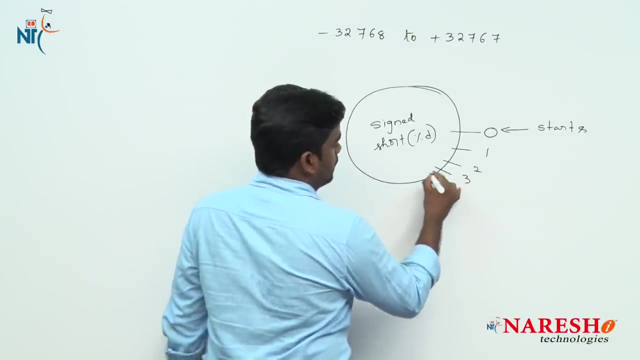 nothing but a percentage d. any value you want to count, either positive value or negative value- starts with a 0.. Counting all the values you want to count- either positive value or negative value- starts with a 0.. Counting always starts with a 0 positive values, counting in a clockwise direction. so 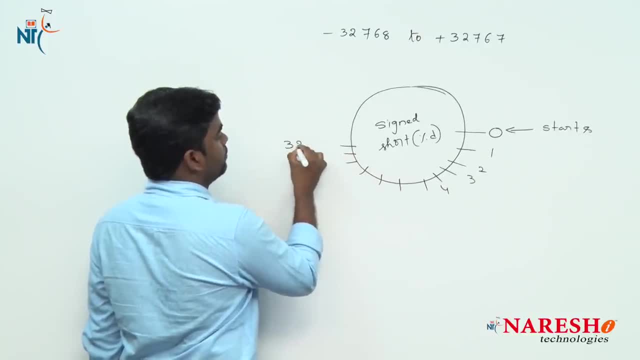 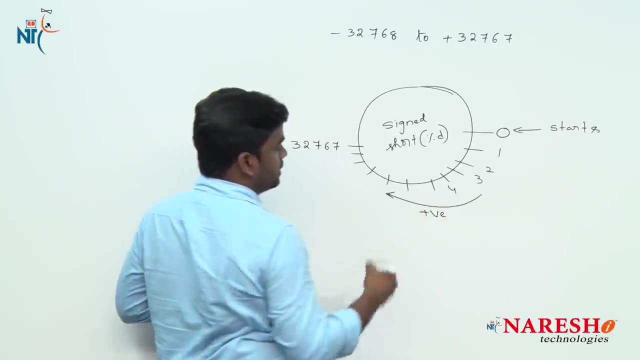 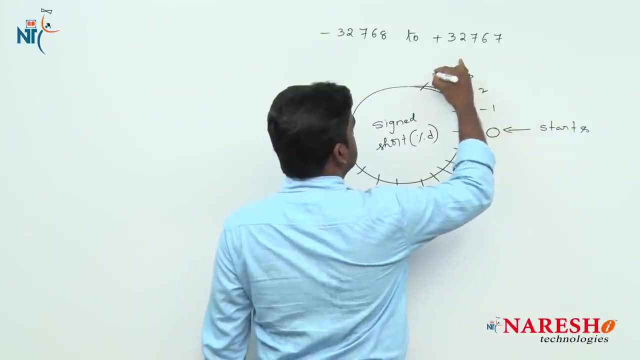 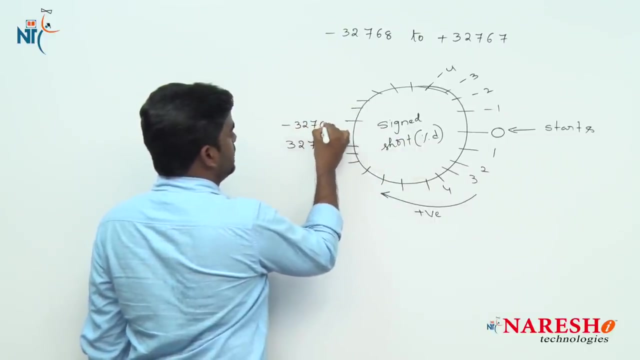 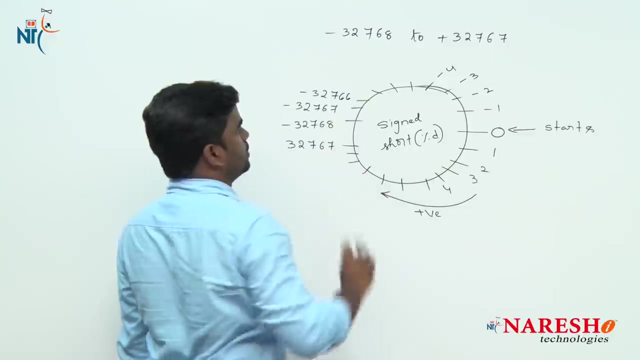 like that and the value maximum value is a 32767. positive values counting in a clockwise direction. remember: Negative values counting in anti-clockwise direction: minus 2, minus 3, minus 4, and so on, Up to Minus 32768, some more. I am writing: minus 326, 7, minus 327 double 6, and so on. 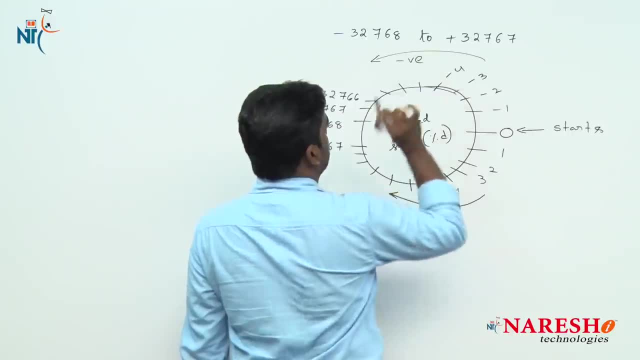 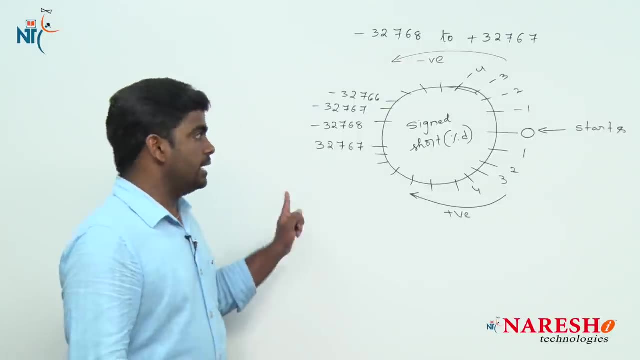 See, these are negative values in a counter clockwise direction or anti-clockwise direction. just limits of a short data type. I have written right in the form of circle. Now, based on this, now we will see some programs on a short data type. observe here clearly: 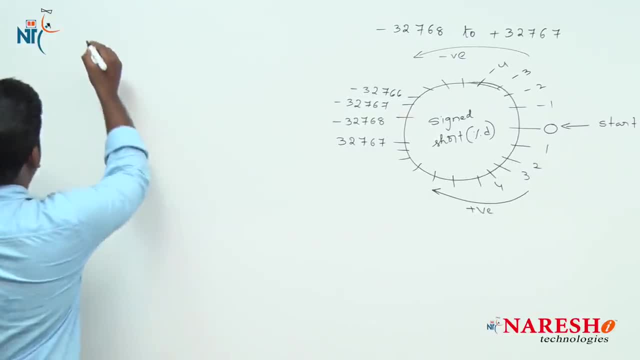 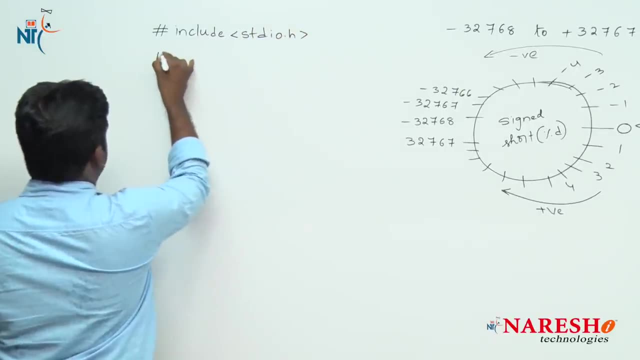 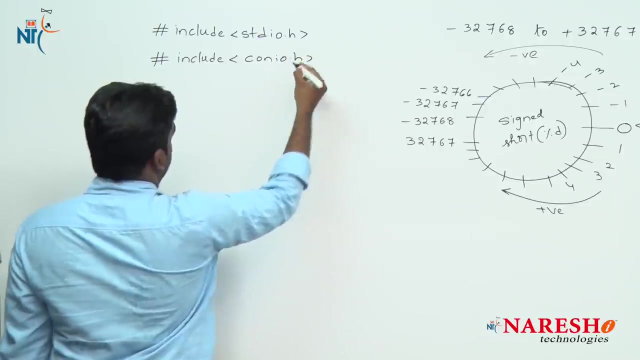 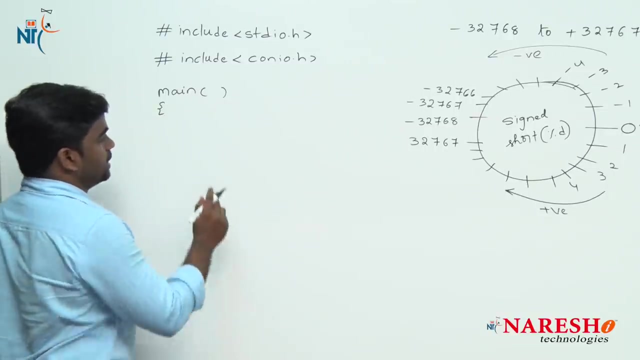 Okay, So now I have written in the form of circle. now, based on this, now we will see some programs on a short data type. hash include header files. I am including stdioh and one more header file, conioh, for clear screen purpose. conioh, inside that main, inside the main, and here it is. we are declaring one. 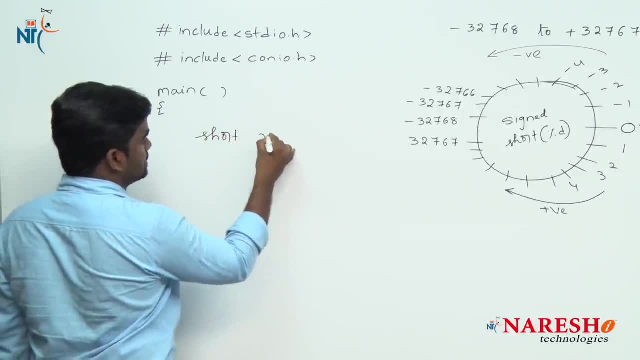 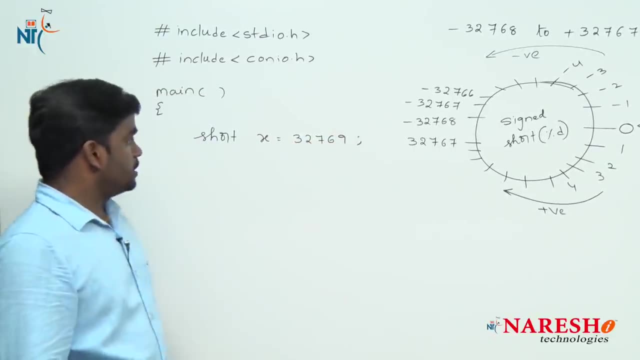 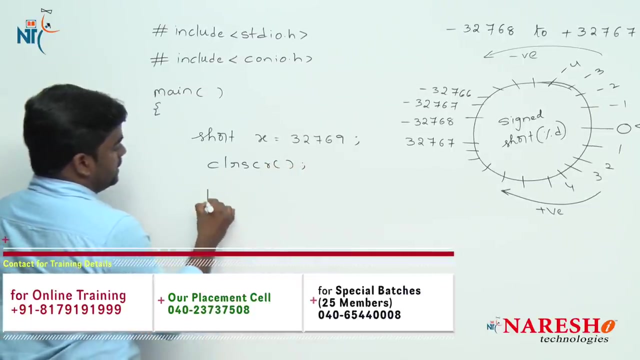 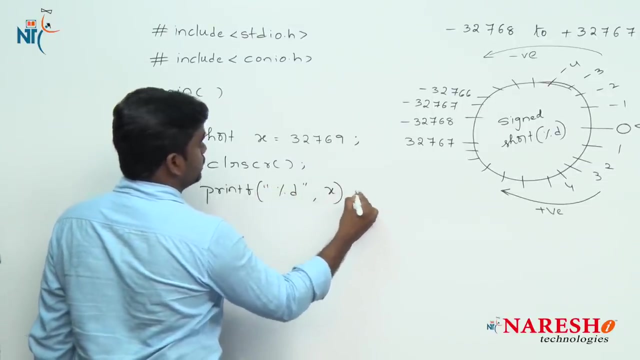 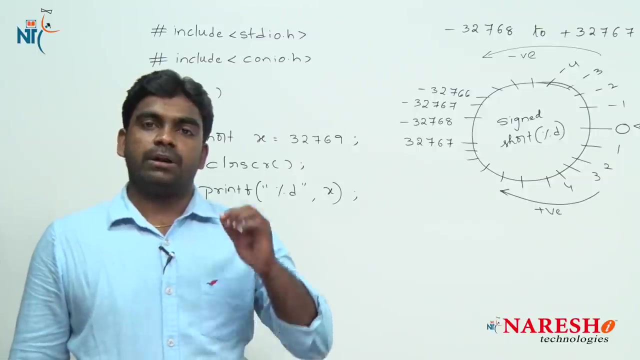 short variable. short x equals to some 32769. we are storing 32769 and here clear screen, clear screen, and we are printing the message: printf: %d, that x value. we are printing. observe here clearly The statements: Executes one by one, from top to bottom. from top to bottom, it will execute, and here it. 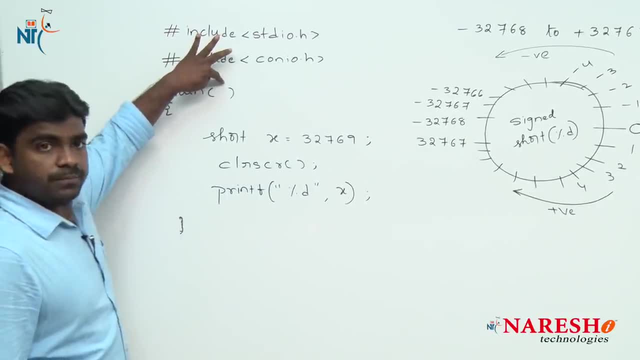 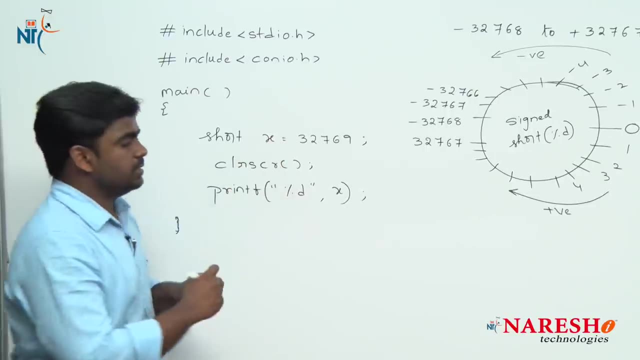 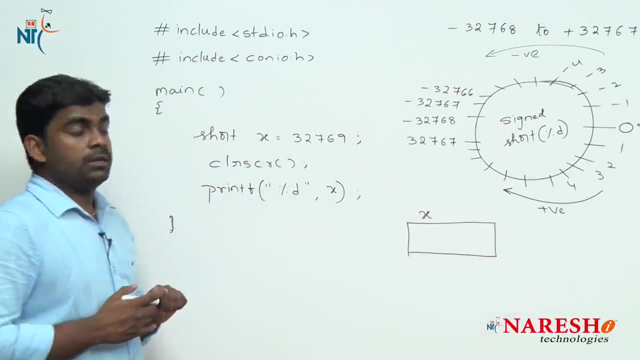 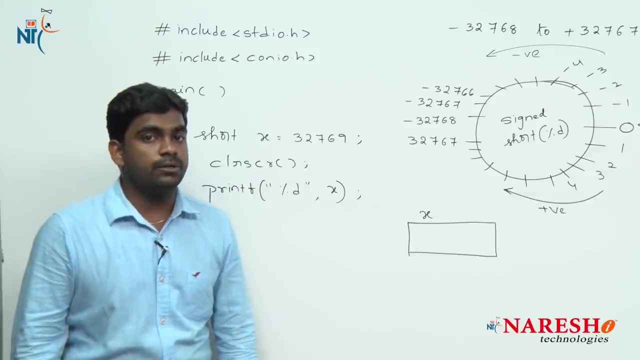 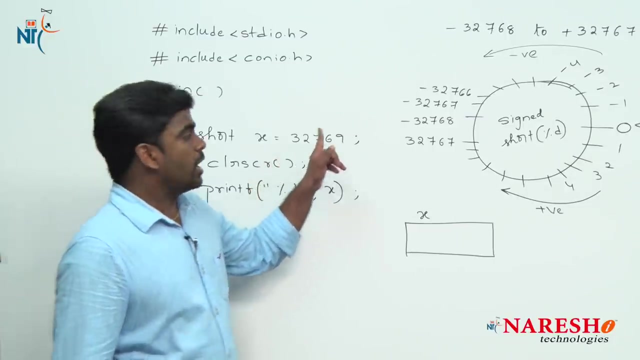 is. execution starts from the main function. the first statement, execution. here it is: x gets memory allocation at any location. x get memory allocation. x get memory allocation, but what is the value you are storing? 32769 is the value you are storing. What is the value 32769 you are storing? so, based on this, it will count. 32769 is a positive. value now. so it starts counting positive values here: 12, 3, 4, 5, 6, like that it will keep on counting 32767, 32768, 32769.. So 32769 value is equals to minus 32769.. So 32769, that value is�. tattoos at where I was started: 2100. So 2 times 1 is equal to 2 times 1. 3 times 2 means 1, 2.. 3 times 1 is Public employee is present. Ruler is 1 and 3 twice by 2 times 0 plus 1, which means this, Elias, is in your packet from. 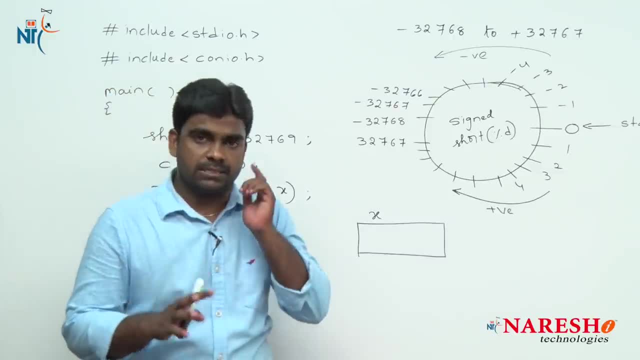 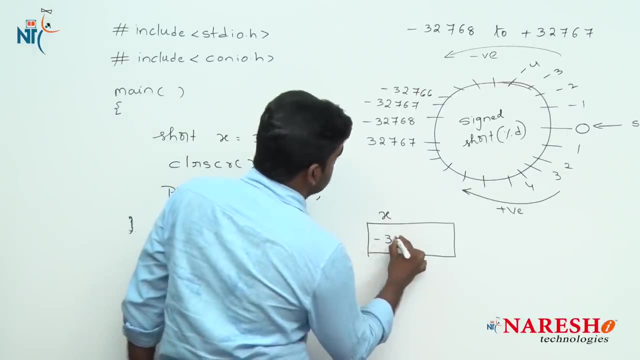 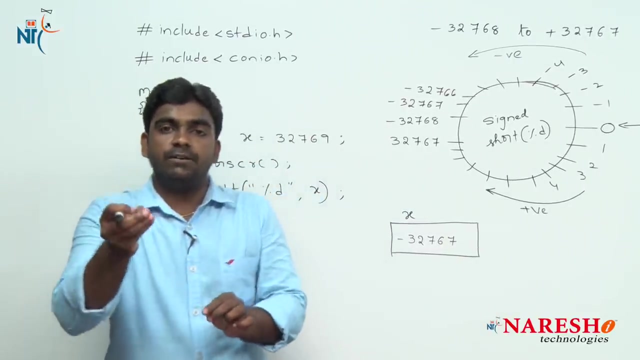 the dochos you are storing value is 1220. what is the value 32769? you are storing. what is the value 32767.. It will not give any error message. It will store one garbage value in the memory. So what is the value Minus 32767.. What is the value Minus 32767 will go and store in the 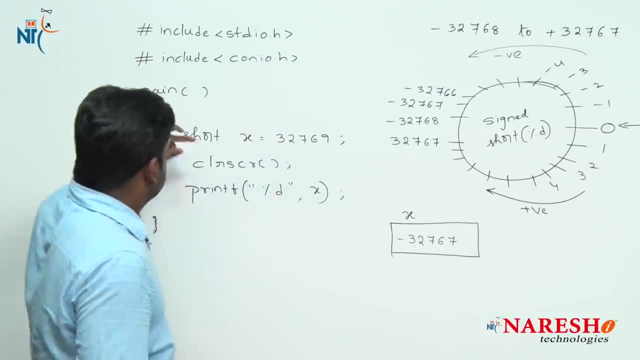 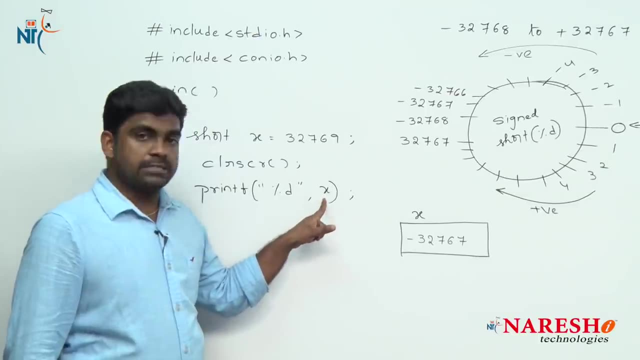 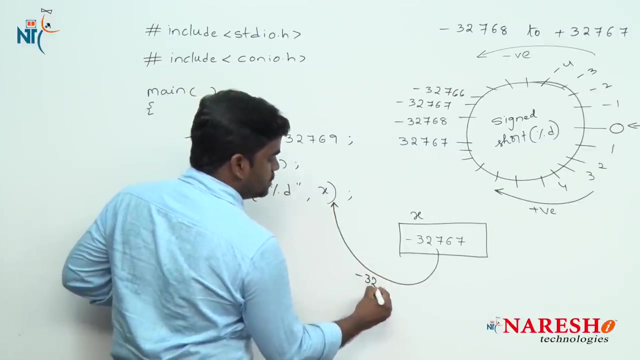 memory: Garbage value. Next it will clear the screen. Next we are printing. So whenever we are printing x value it has to collect. So from this it will collect that x value. What is that x value? Minus 32767 is a x value. It will fetch that value From where? From the memory. 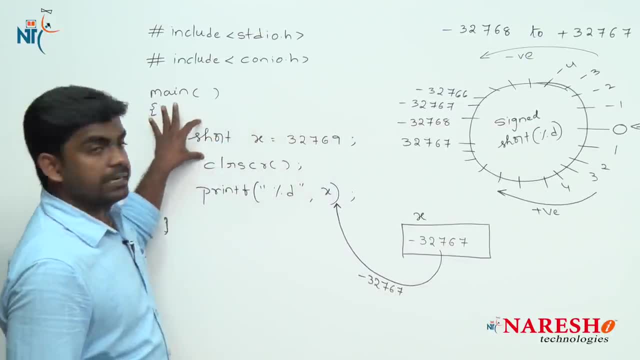 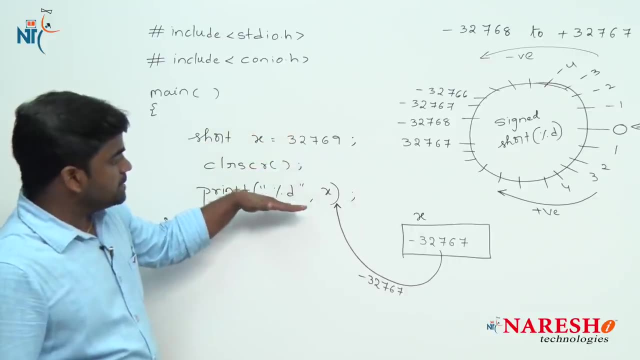 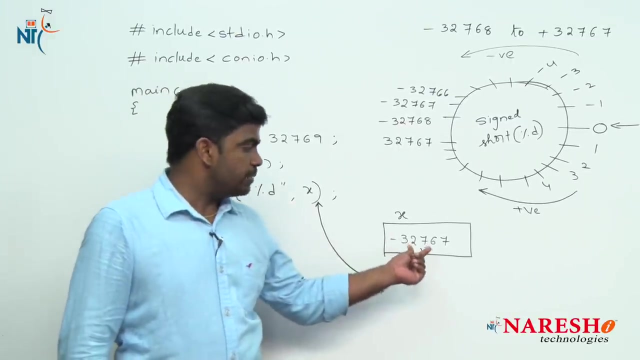 It will not look at the declaration area. Declaration statement: already completed. Throw out No use. Next we are at the third statement. We are printing The x value. We are printing the x value. So what we are printing: Minus 32767, we are collecting. 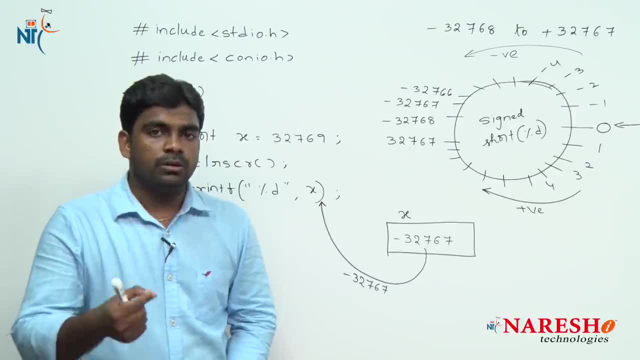 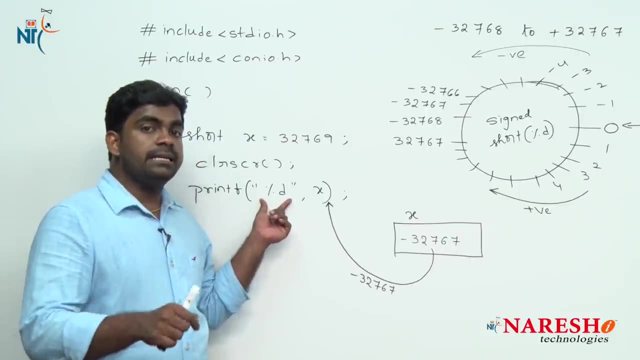 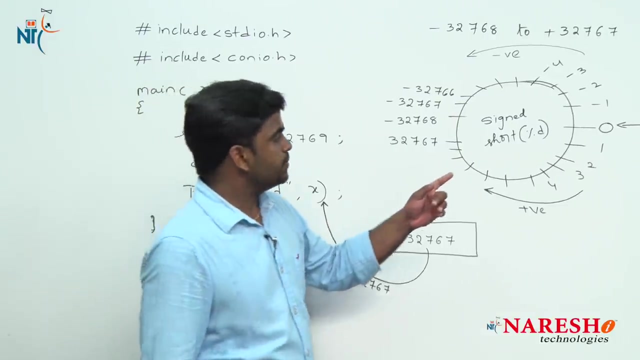 But it will not print directly What it will do According to the format specifier. What format specifier you have given Percentage D, you have given So percentage D circle. it will check. Sir, where is the percentage D circle? Here it is. This is percentage D circle In this. 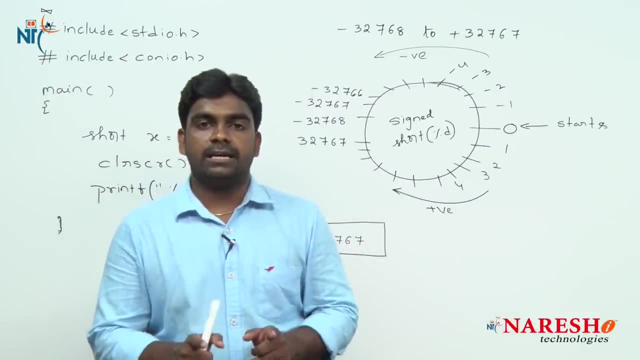 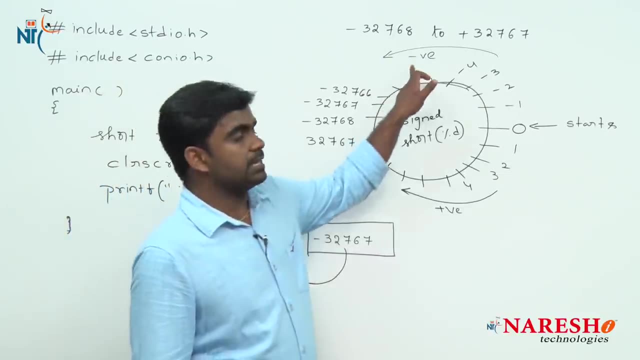 circle the value is present or not. it will check What is the value Minus 32767. value is present or not. it will check in this circle. Yes, minus 32767 is there, So it will print the value. 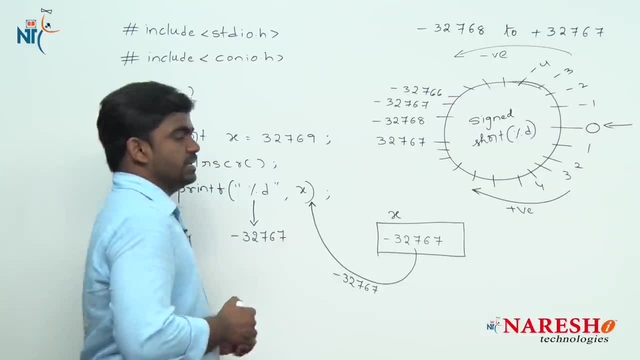 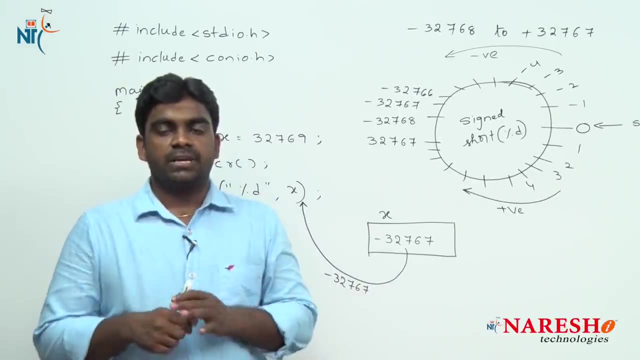 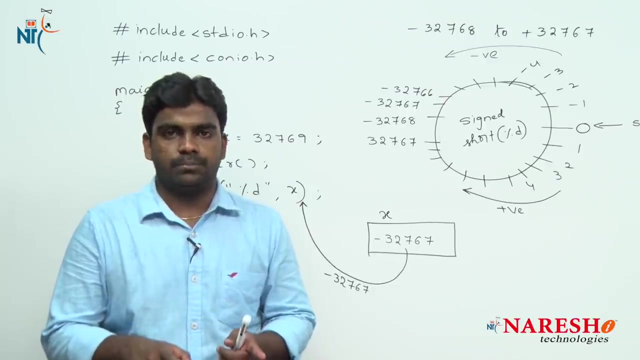 Output is a minus 32767.. Sir, here we are violating the rules. Will it give any error messages? No error messages. Yes, it will store one garbage value into the memory. remember, right, that we should understand because we are doing the mistake. So we should analyze, clear, right. we will see one more program, see here. 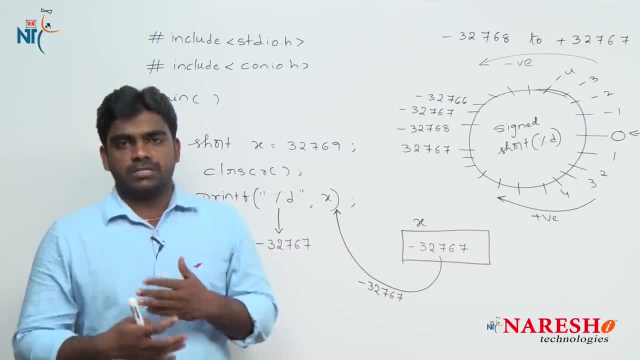 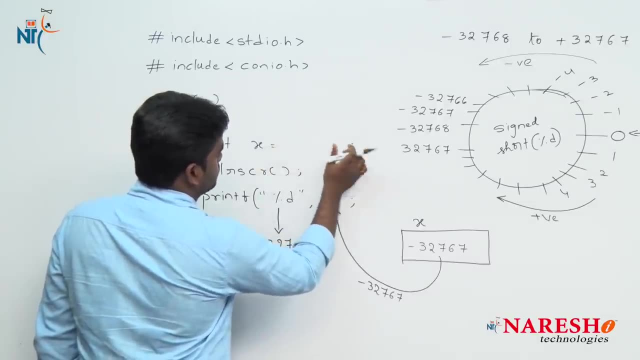 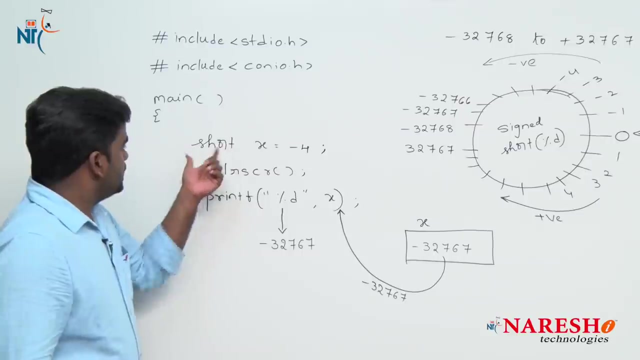 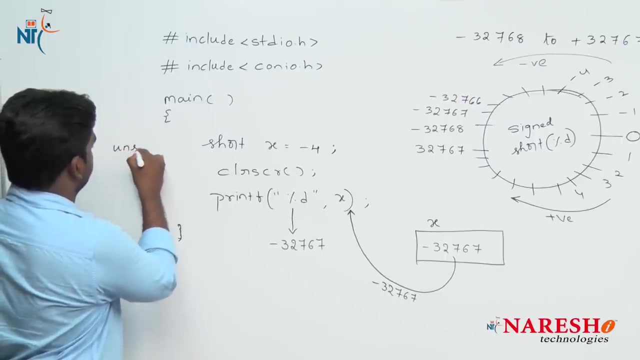 it is a just like a this program, So we will see some more complex programs. ok, see, suppose now I am changing that x value, x value to minus 4, x value to minus 4, but here it is explicitly, I am specifying very clearly that this is unsigned short integer. unsigned short integer value x. 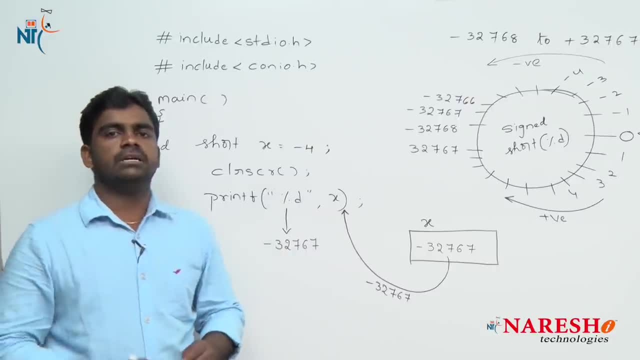 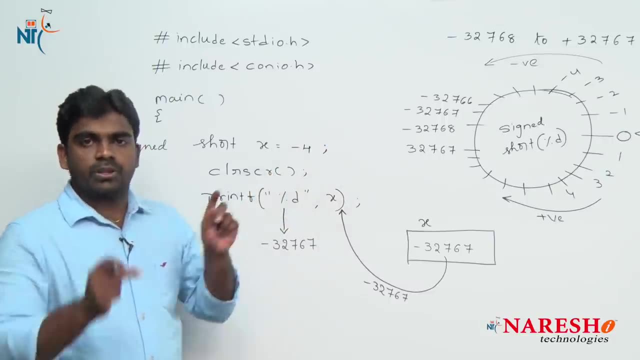 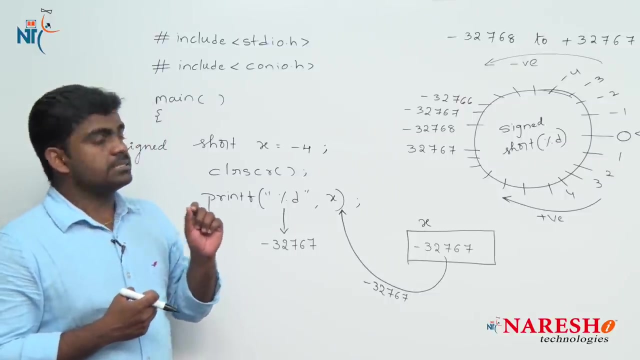 value, but I am initializing with the value 4.. Sir, actually unsigned will take only positive values. now, yes, but here it is. Whenever we are trying to assign the negative value according to that circle, sir, what is that circle? now we have to discuss about unsigned circle also. So, unsigned circle, we are writing. 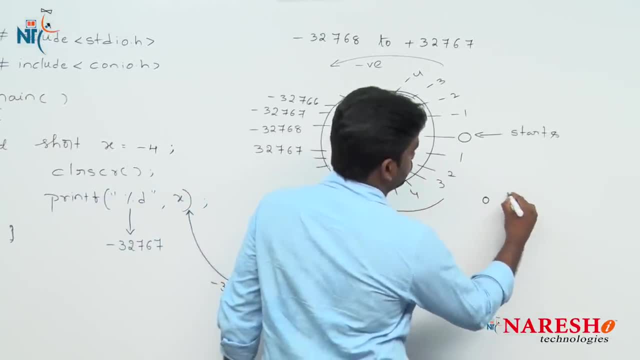 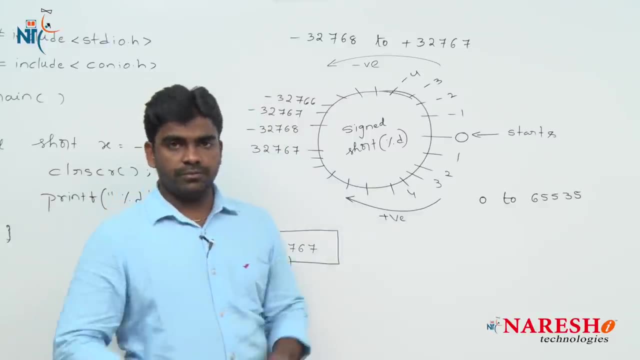 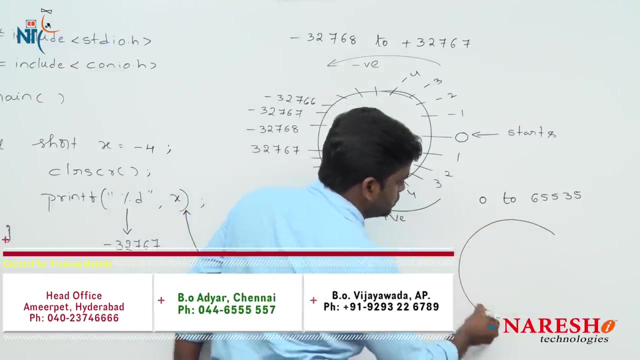 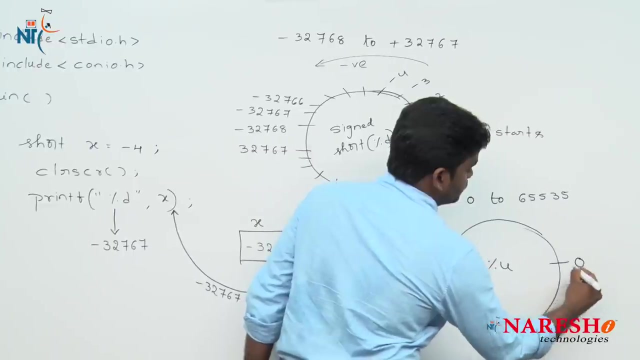 first, the value is a 0 to 65,535. this is unsigned range. we discussed already 0 to 65,535. I am just writing in the form of circle, same values. This is percentage. u is unsigned circle and here it is a counting. starts with a 0 only positive. 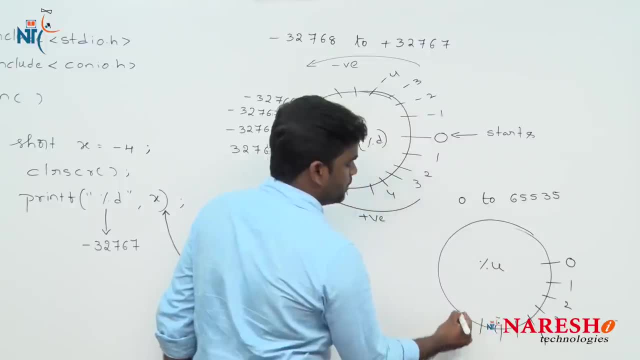 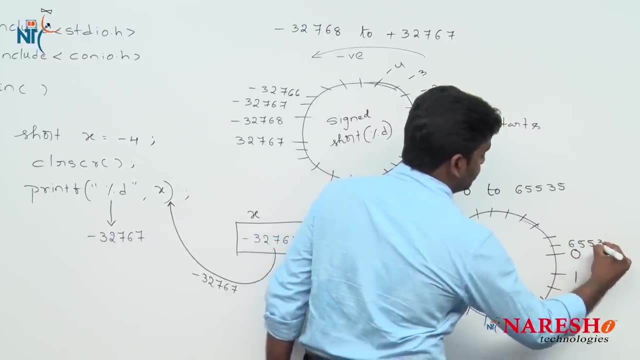 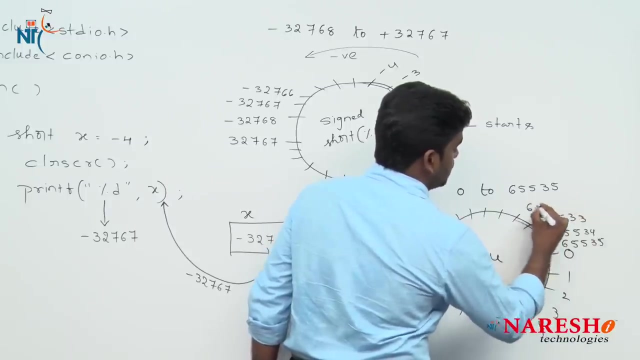 values are there: 3,, 4 and so on and so on. what is the maximum value is a 65,535 and some more values: 6,, 5,, 5,, 3,, 4, 6,, 5,, 5,, 3,, 3,, 6,, 5,, 5,, 3,, 2 values we are writing. So this is a range. 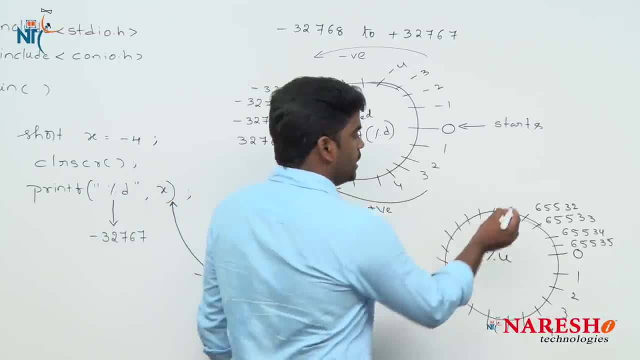 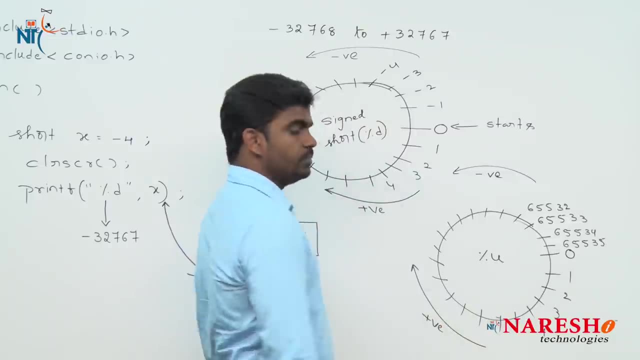 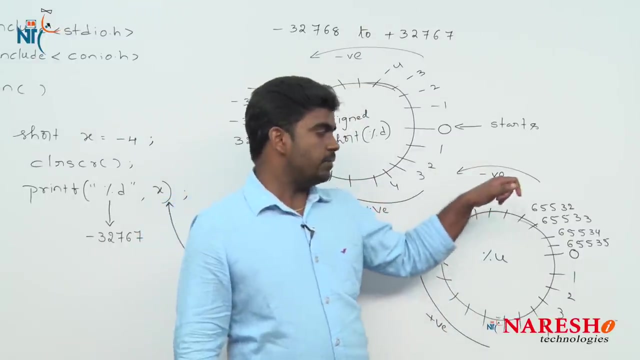 Just this. we are writing that range in the circle, same story: negative values counting in a anti clockwise direction, positive values counting in a clockwise direction. One is a clockwise direction and second, one is a counterclockwise direction. right, positive values counting and negative values counting. So here now I am trying to store the value minus 4.. 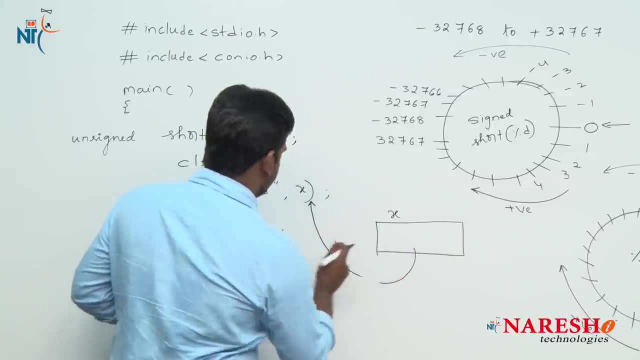 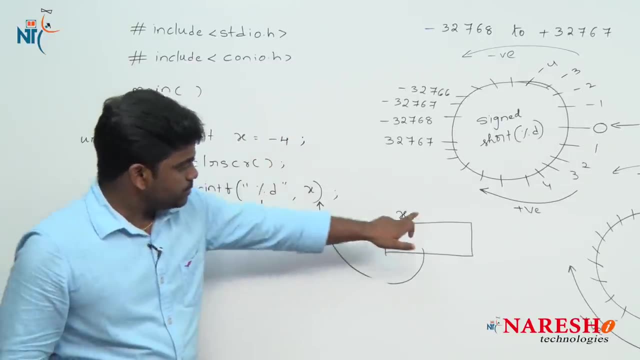 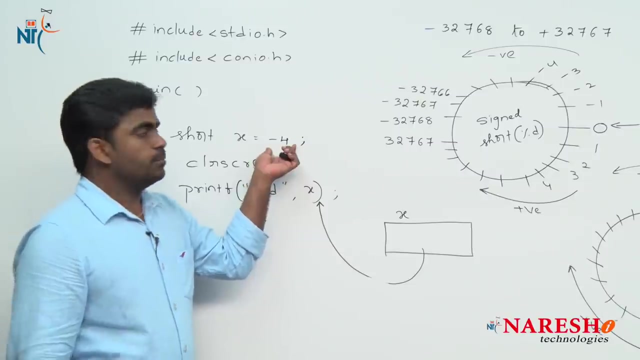 So, as usual, first x gets memory allocation, x get memory allocation. x value is a minus 4 right, first x memory will be allocated. x memory will be allocated but it has to store the minus 4 value. but what we have given unsigned you have given. So in which circle? 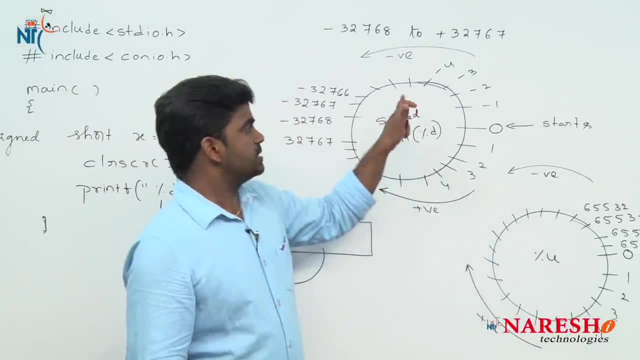 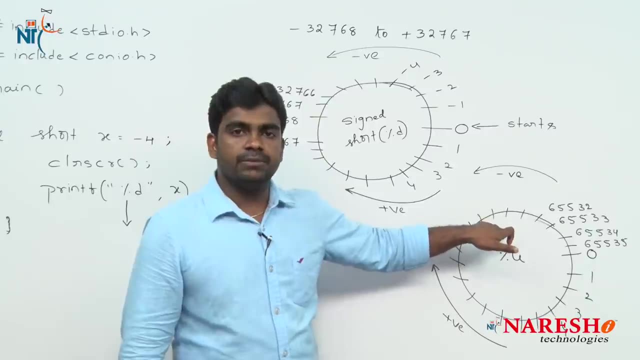 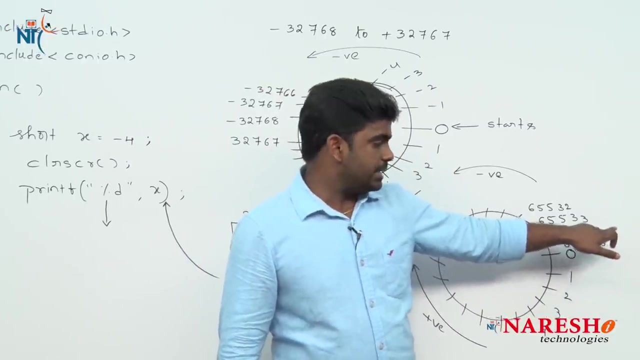 it will check in this circle or in this circle. this is a signed circle and this is unsigned circle. So in this circle it will check. in this circle it will check. So here it is. we need to count that minus 4 value. minus 4 is a negative value. So minus 1, minus 2, minus 3, minus 4, minus. 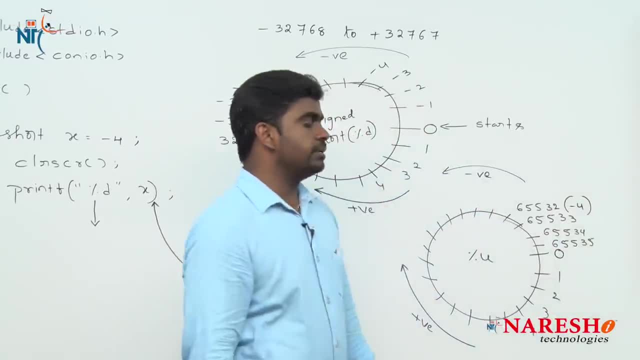 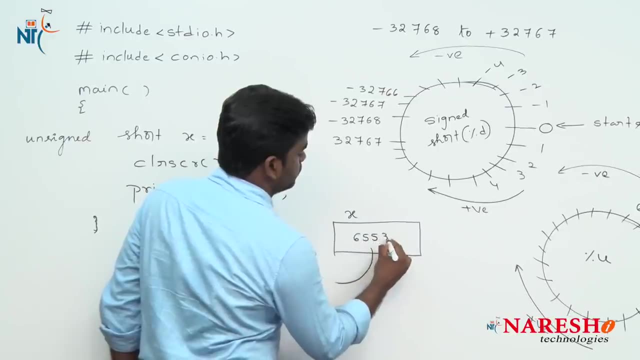 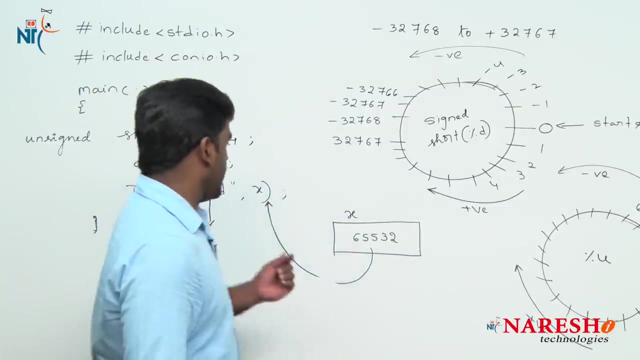 4 value is equals to 6 double 5, 3, 2.. So in the memory, so what value will go on store is a 6 double 5, 3, 2 will go on store. 6 double 5, 3, 2 will go on store. and now here, So we are printing. 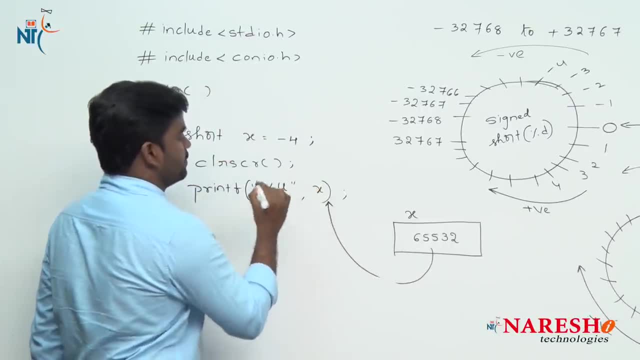 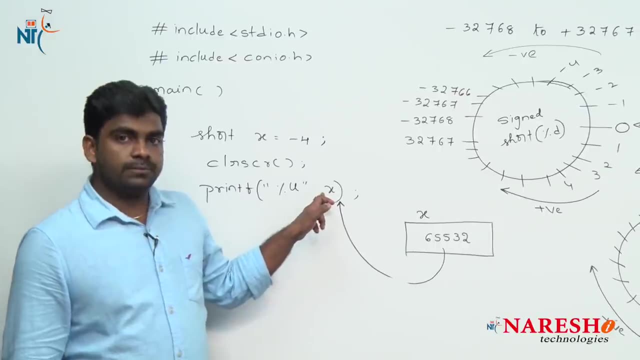 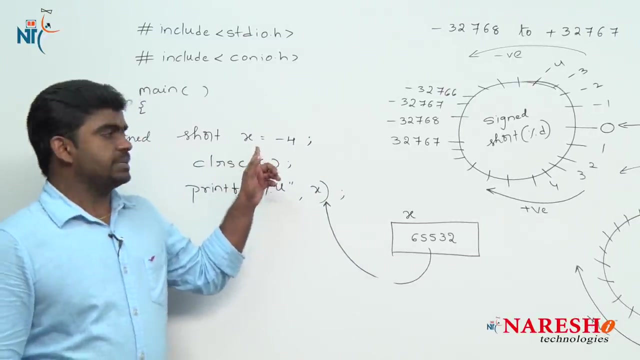 percentage u. What is a format specifier? I have given percentage u, I have given percentage u, So first it will fetch that x value. So what is that x value? please do not look at that first statement in this program, because first statement is used to allocate the memory only. Once you allocate the memory from 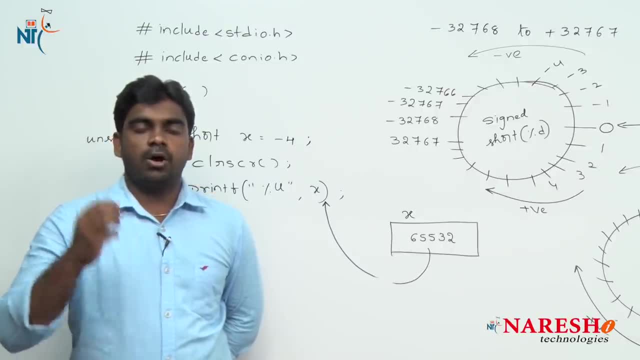 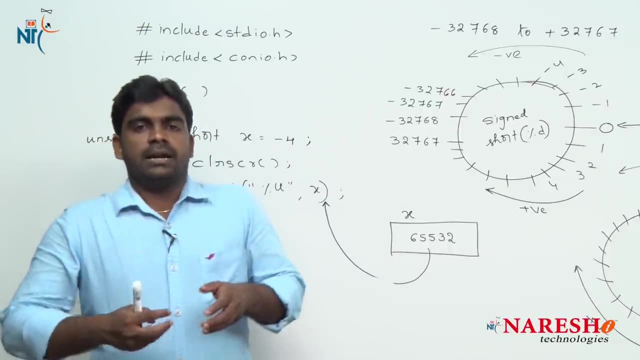 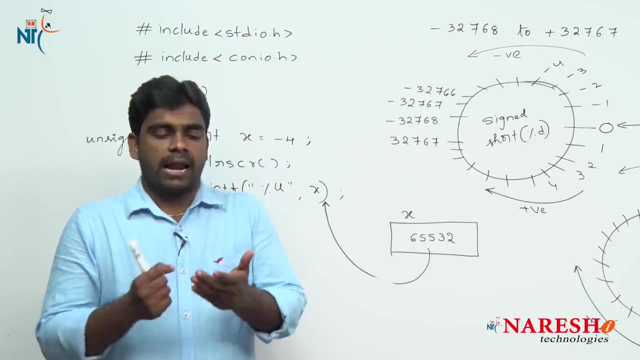 the second statement: wherever you use that variable, always it will collect the information from the memory. only the best example thing generally. For example: right, I just deposit some amount- 8000 rupees- into my account today. right, I visit the bank and I have to write one receipt right for payment and bank management first will. 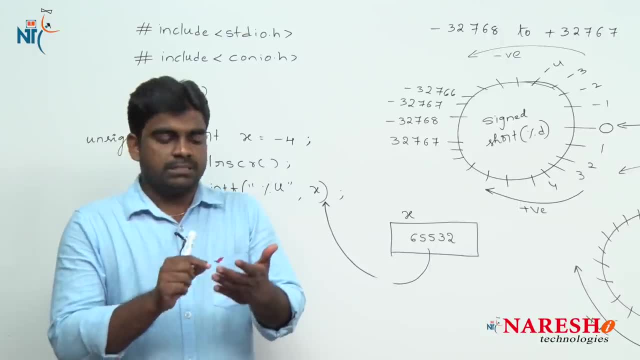 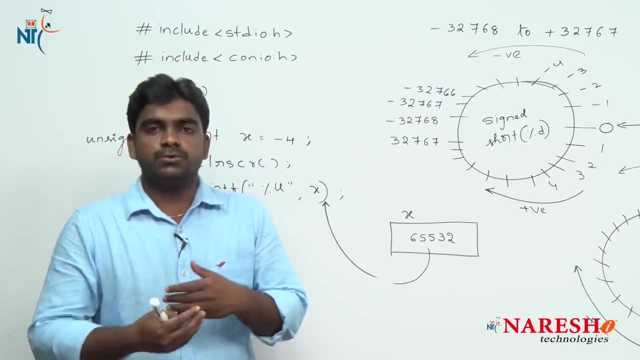 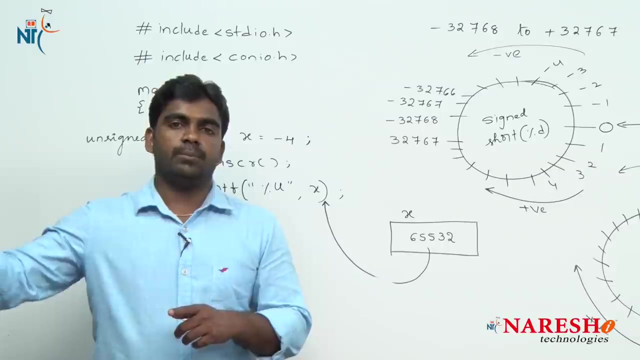 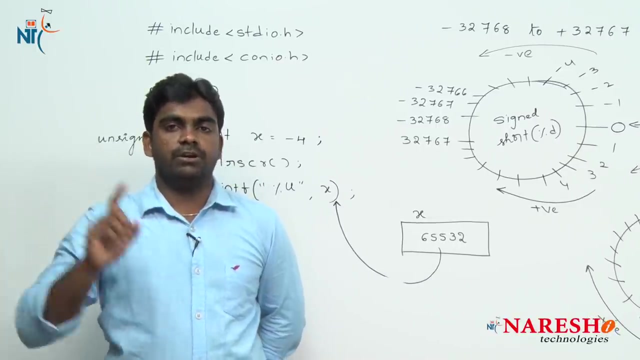 follow that receipt to perform the transaction by just look at that receipt. So they will deposit 8000 rupees into my account the next day. I just want to withdraw 5000 rupees. bank management will follow. the concept is later on. So they will collect that information from the memory they will. 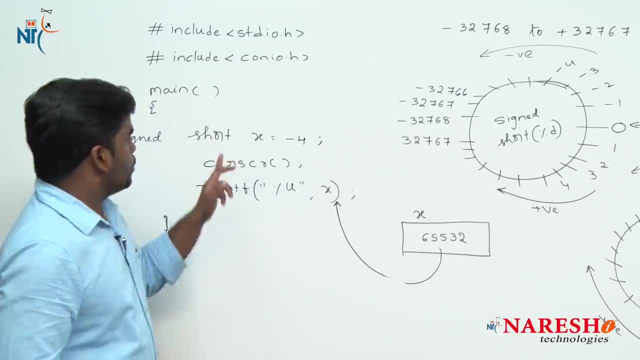 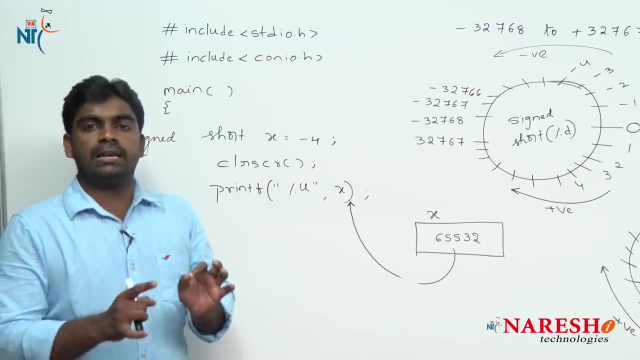 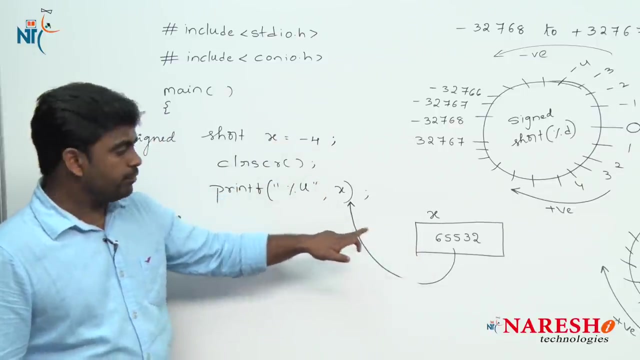 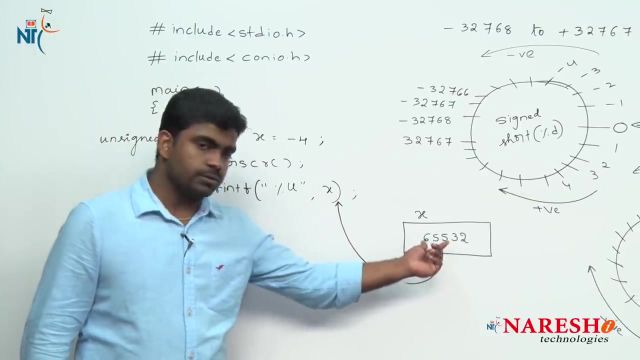 not maintain the receipts in the same way. So once you declare the variable, once you declare the variable in the first statement, which is used to allocate the memory only, once memory allocation has been completed from the second statement it will follow the memory only. So whenever you are printing x value it will fetch that x value: six, double, five, three, two. 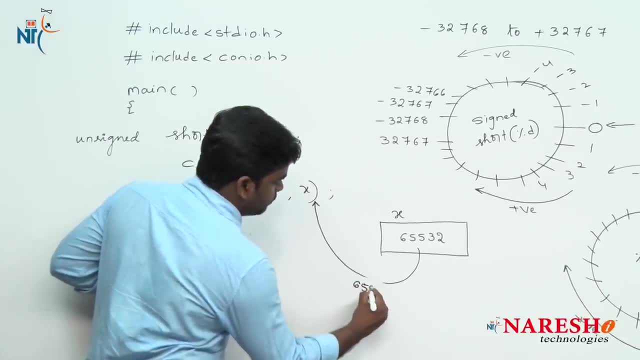 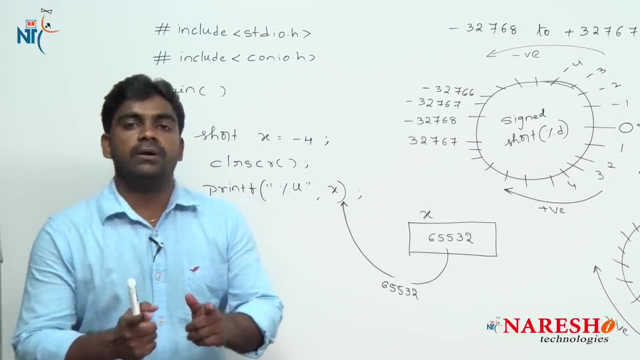 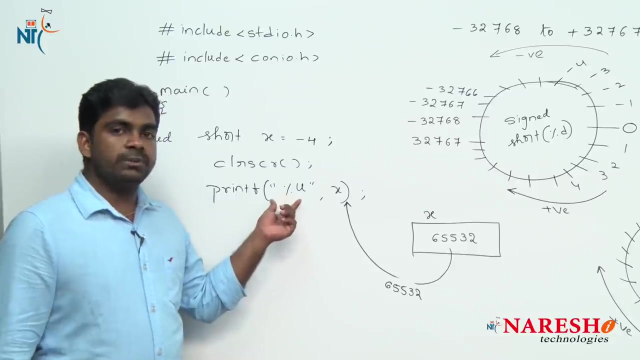 it will fetch. So it will collect that six, double, five, three, two and directly. it will not print again. it will check what format specifier you have given. what is the format specifier percentage u you have given. So percentage u means what in this circle it? 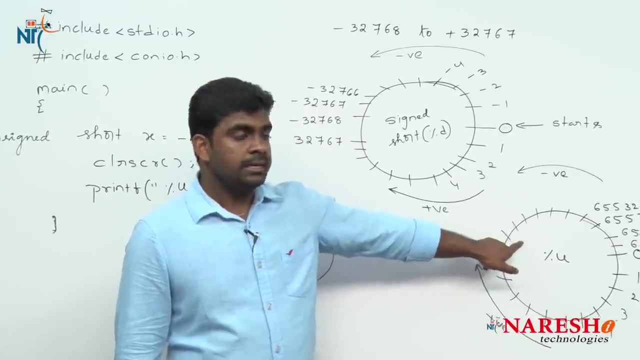 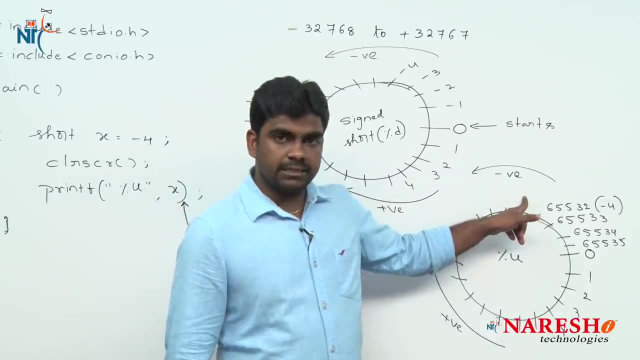 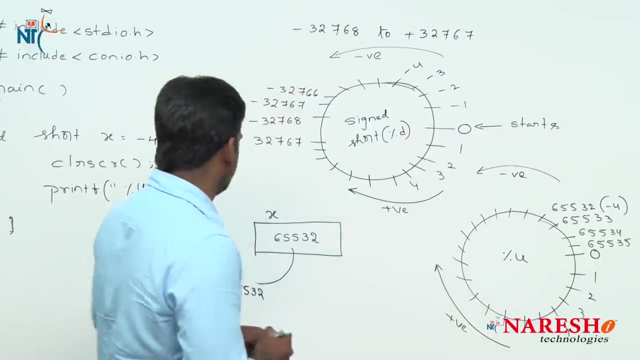 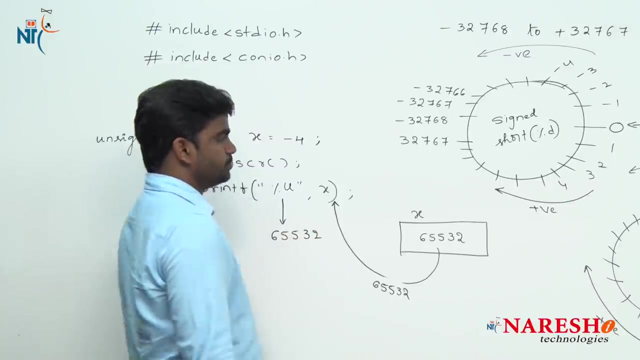 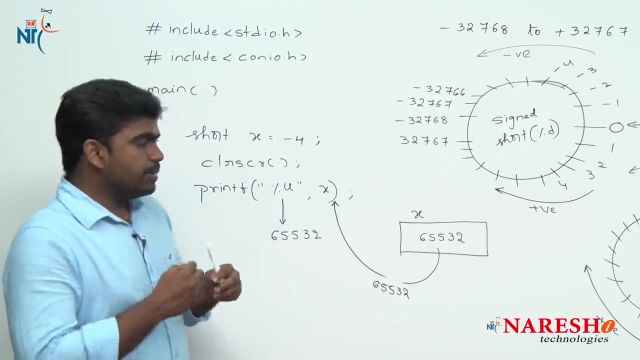 will check percentage: u circle. in this circle 65532 is present or not right, Suppose if it is a present right. So then it will print that value: yes, is there? 65532 is present. So in the output, in the output it will print that message: 65532, 65532. it will print remember and see, for example: 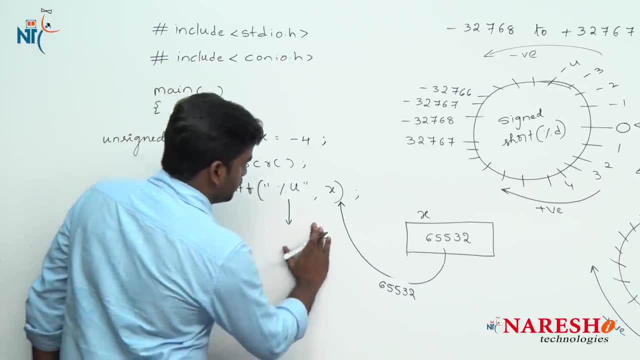 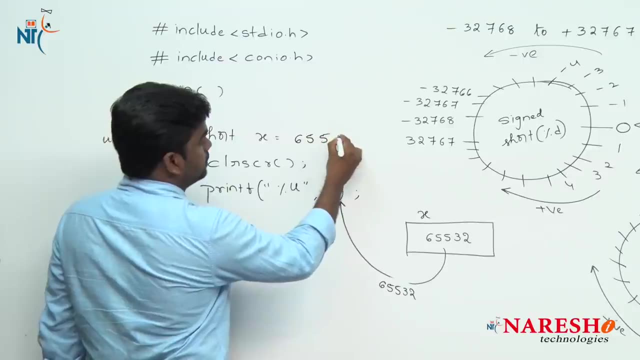 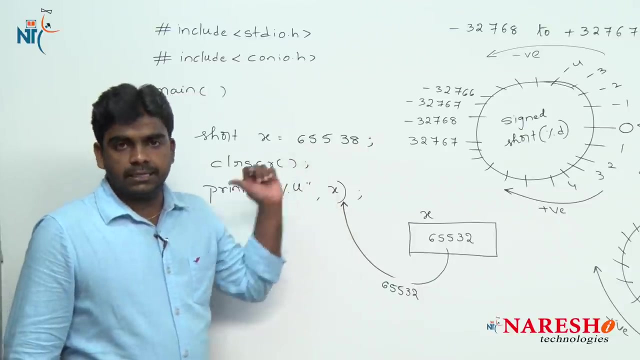 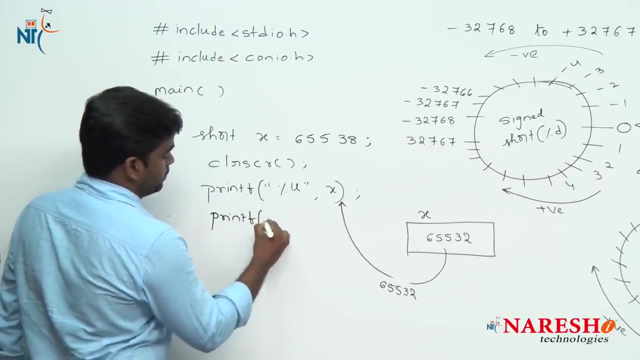 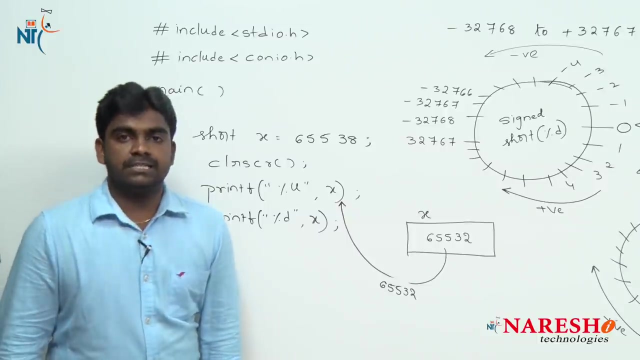 one more thing we will see. this is unsigned value only, but I am printing 65538. we are storing Now the value is 65538 and we are printing %ux. and one more. we are printing printf: %dx, %dx. Now observe the concept. what value will go and store into the memory is first. 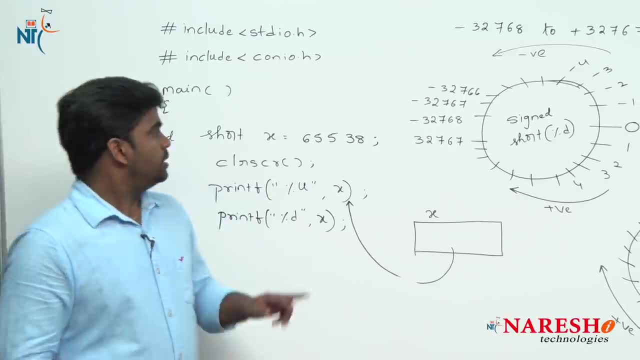 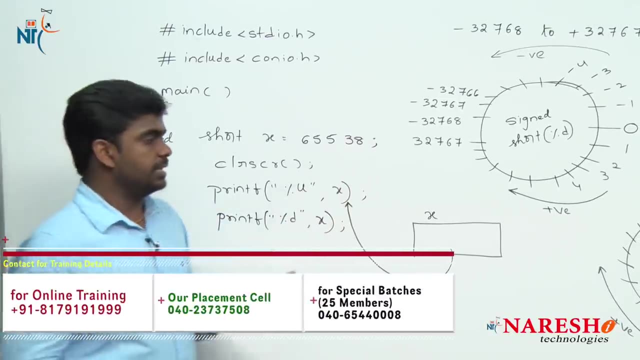 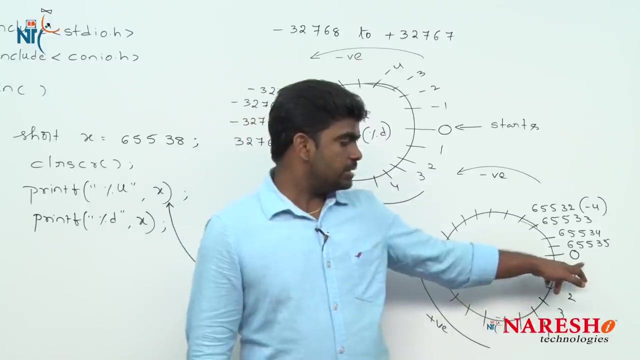 in the memory what value will go and store. So you have given unsigned and the value is a 65538.. So in which circle it will check? in the second circle it will check. in the %u circle it will check. So it will start counting 0, 1, 2, 3, 4 and keep on counting 65538. 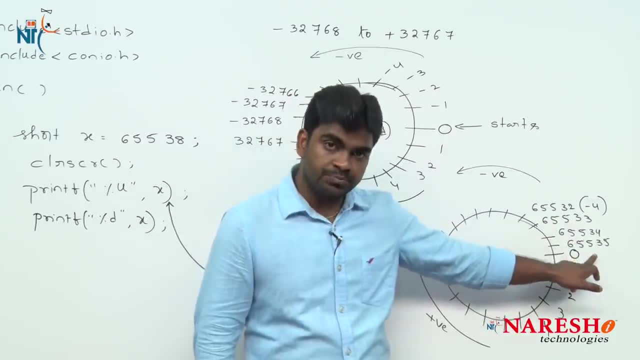 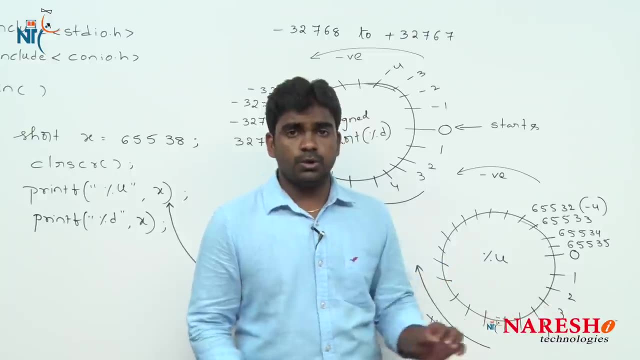 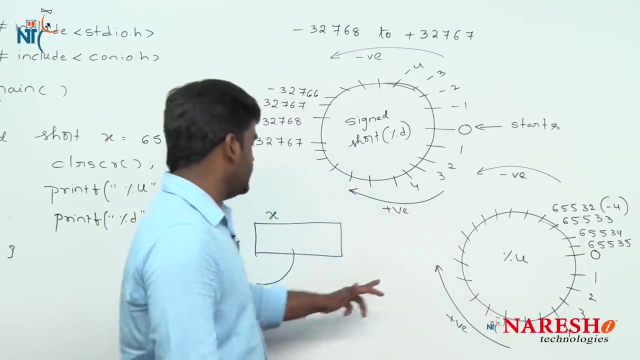 365, 3565536655366553765538.. So lif очерiring 15кон살 lal 69538. value is equal to 2, is equals to 2.. So here it is in the memory, the value. 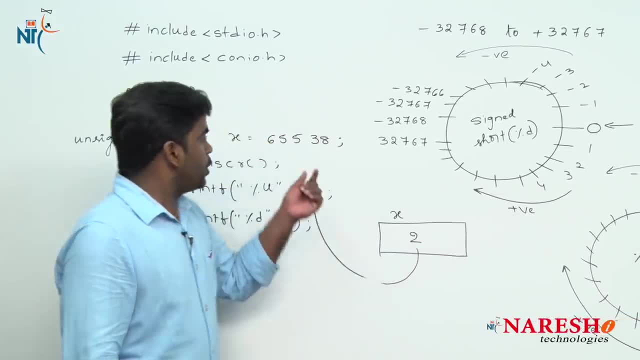 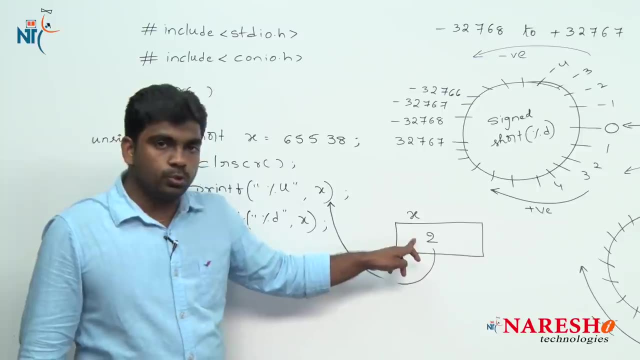 2 will go and store. It will not store 6 mile, 53 a right. So while counting in that circle the value 6, Double, five, three, eight is equal two, five, three, six, six, five, three, five, four, six, five, three to 2 right. So in the memory now 2 is there. So first statement completed. Next is control. 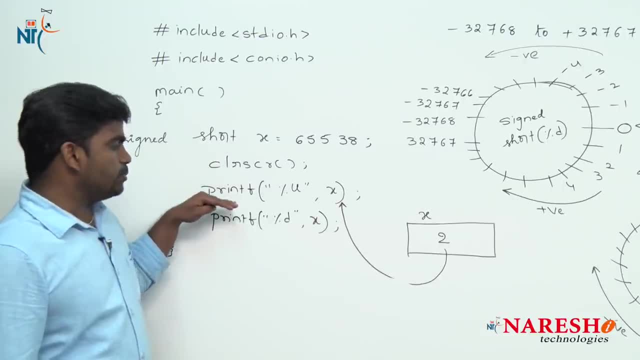 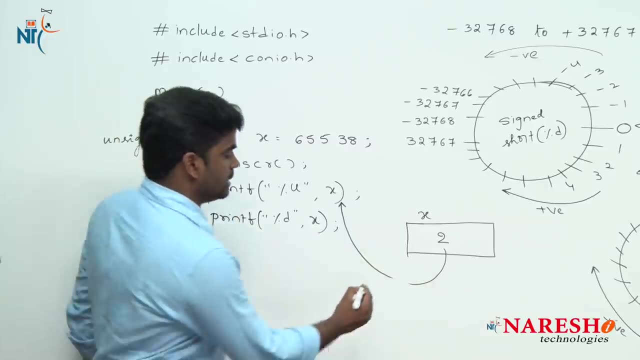 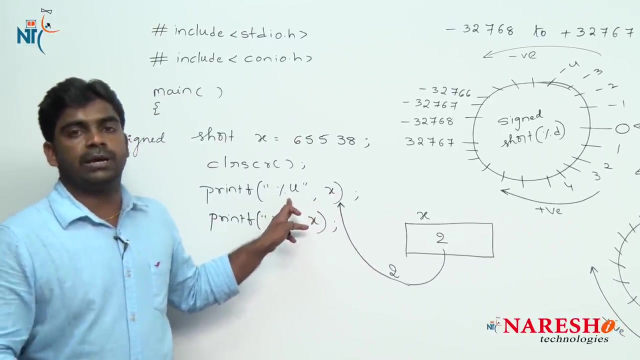 come to that second statement: clear screen and next that control. come to that third statement. we are printing x value. What is the x value 2? It will collect that value 2. and here it is: what format specifier you have given, percentage u you have given. 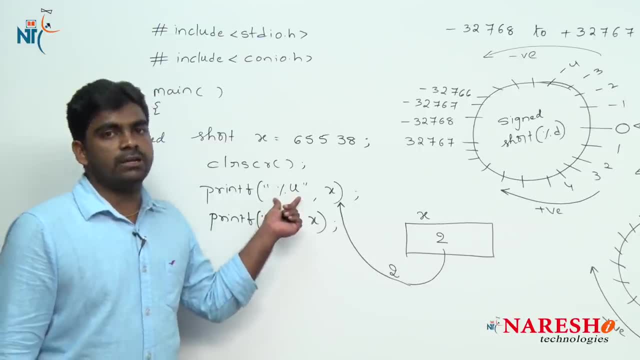 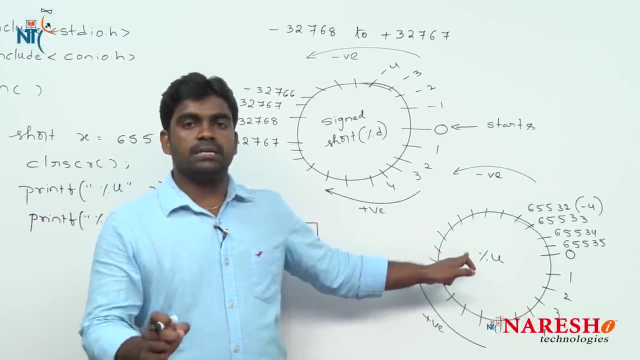 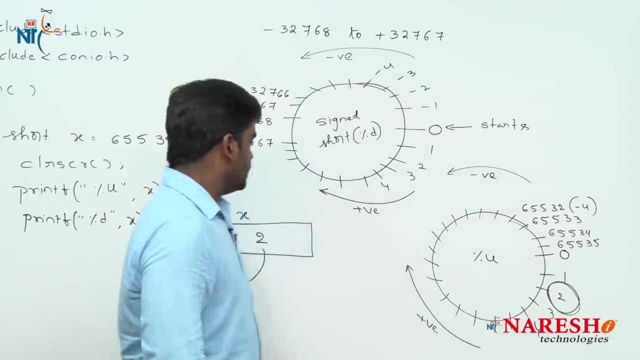 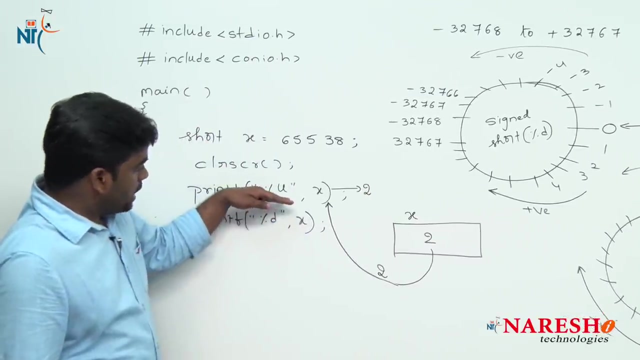 What is the format specifier? Percentage u you have given right. So percentage u circle. it will check in this circle the value 2 is present or not. Yes, the value 2 is present. value 2 is present, So directly it will print the value 2. output is a 2 here. Next the control come to that. fourth. 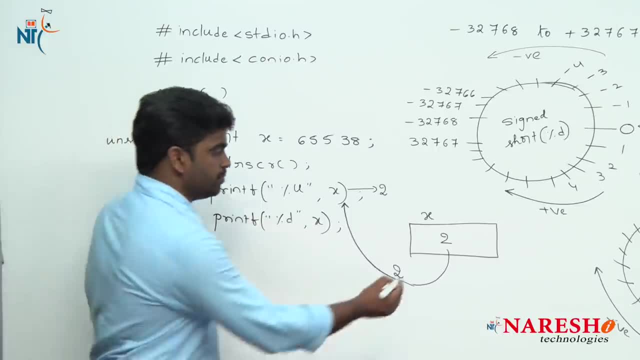 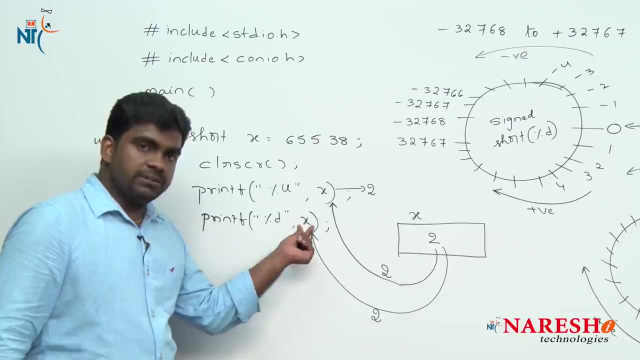 statement again. it will fetch that x value from the memory. Here it is. It will collect that x value from the memory. that is 2 and next format specifier. it will check What is the format specifier. now, Percentage d is a format specifier, So we need to check in the. 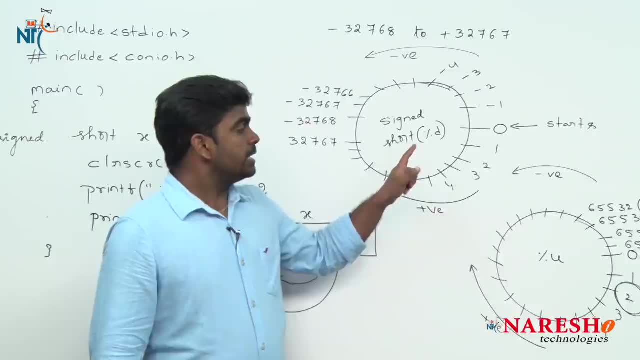 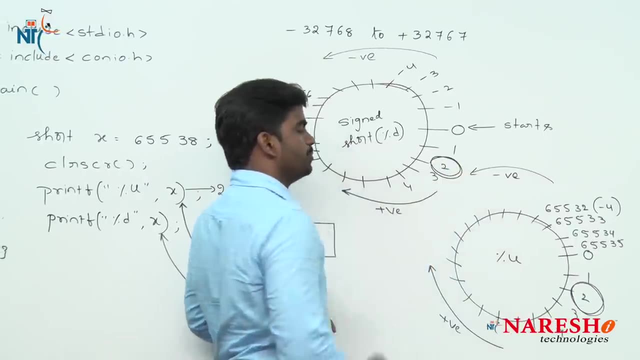 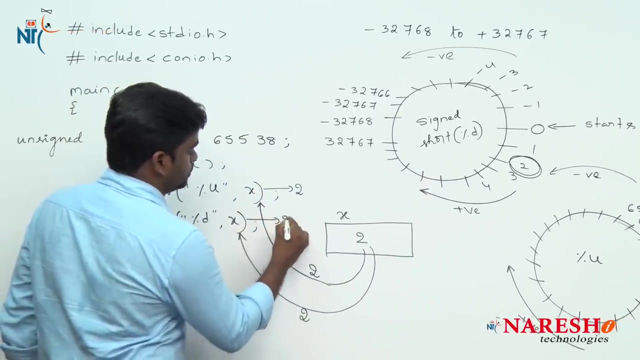 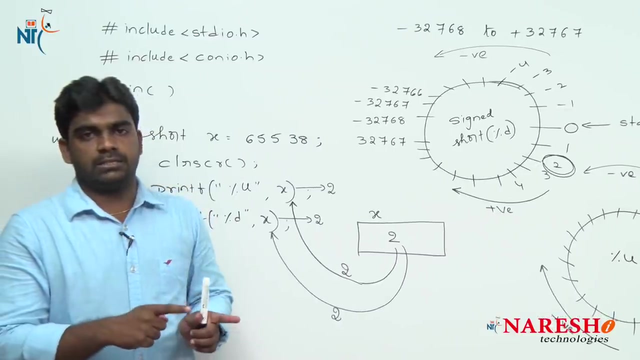 signed circle. This is a percentage d circle. In this circle 2 is present or not? Yes, of course, here it is. in this circle also 2 is present. So here also it will print the value 2.. It will print the value 2, that is it. So we will see one last example. just look at this. 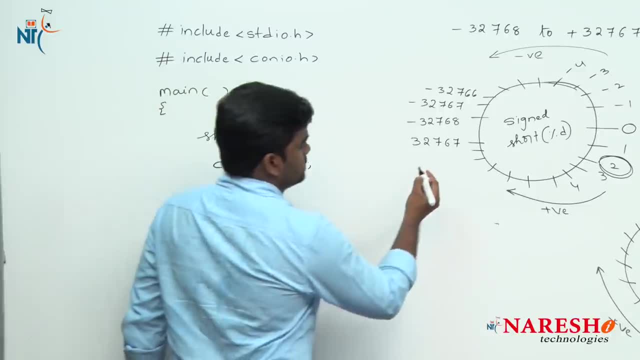 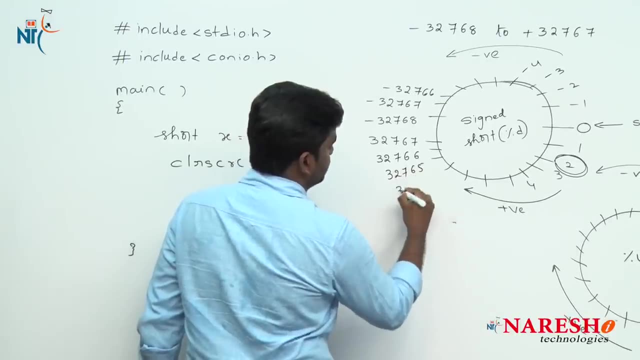 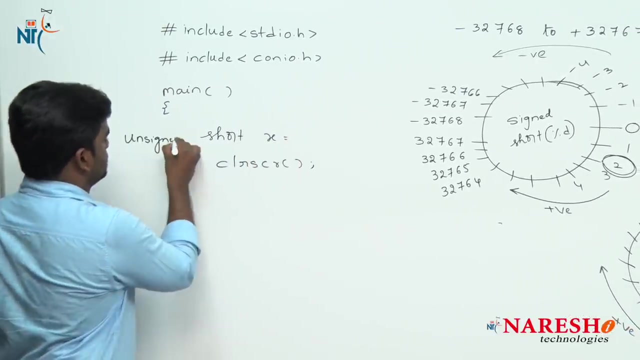 See that example. Suppose, here I am writing some more things. this is 3, 2, 7, double 6, and this is 3, 2, 7, 6, 5, and this is 3, 2, 7, 6, 4, 3, 2, 7, 6, 4.. Now here, unsigned, I am declaring the value minus 3 to. 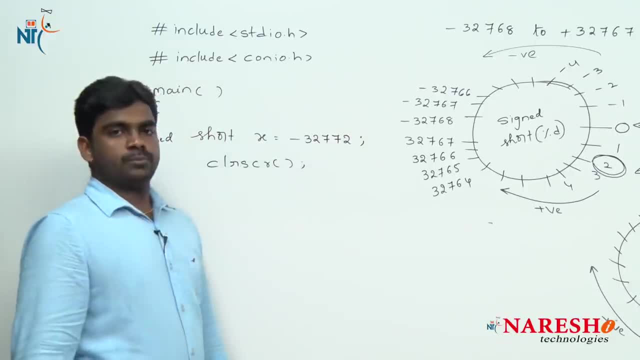 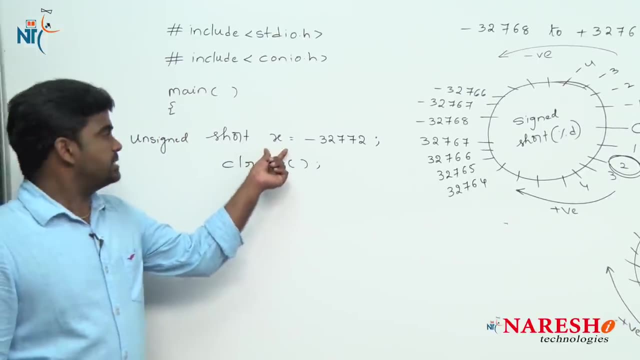 7 7, 2. this is the value I am storing: 3 2 7 7. 2 is the value I am trying to assign into variable x. but x is of type? what Unsigned, remember? and here it is. we are printing that value. print f. 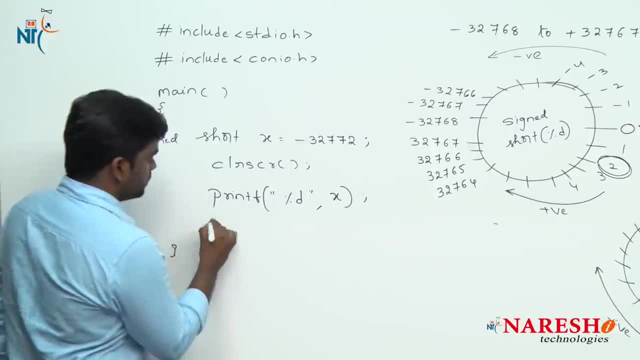 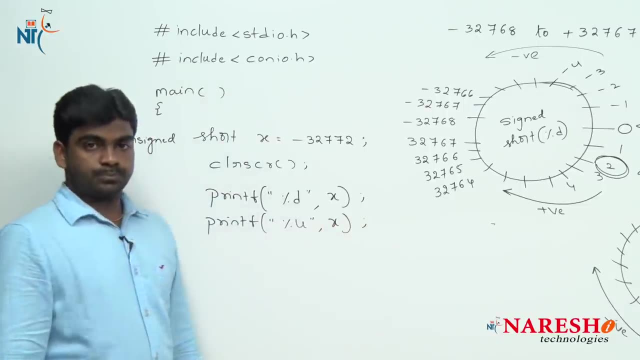 percentage d x value. we are printing and once again we are printing that x value, but I want to change the format specifier. that is percentage u. 3, 2, 7, 7, 6, 5, 3, 2, 7, 6, 4, 3, 2, 7, 7, 2. this is the value I am turning. 3, 2, 7, 7, 2. this is the value I am. 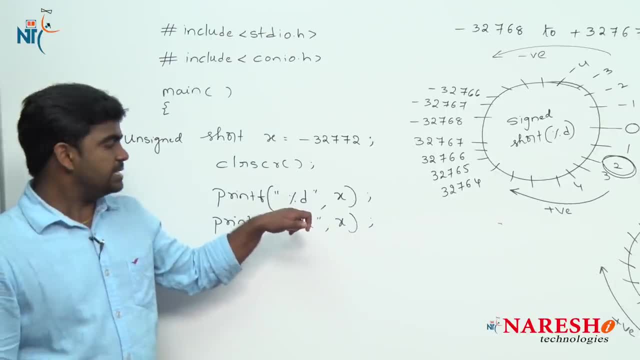 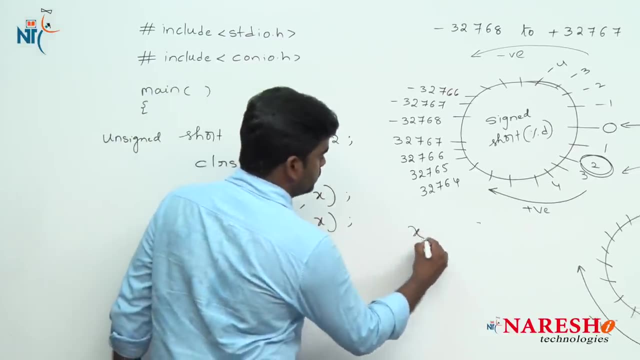 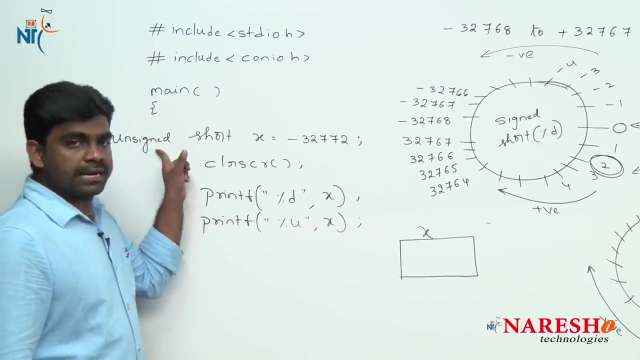 printing two times. First time we are giving that percentage D and second time we are printing the percentage U. But sir, what value will go and store into X first X get memory allocation at some location. What value will go and store unsigned? Unsigned value minus 32772.. So 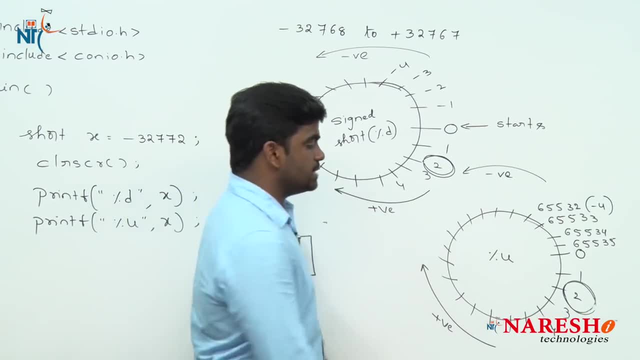 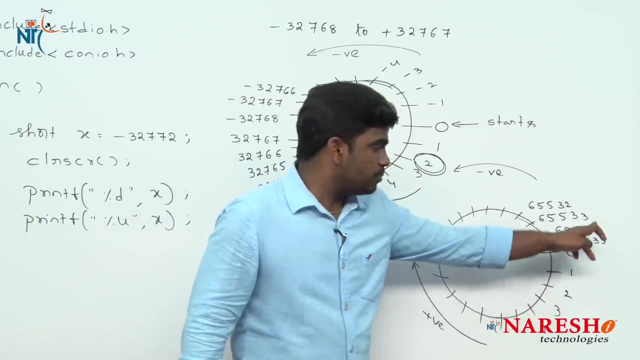 in a unsigned circle. minus 32772, you have to count. Minus 32772 is a minus 1, minus 2, minus 3, minus 4.. Like that, minus 32772, you have to count. Sir, it is a headache na. Yes. 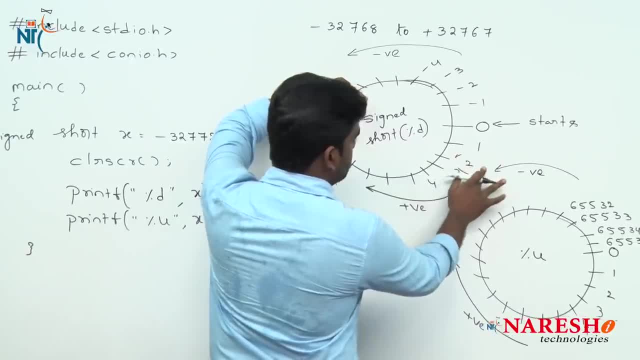 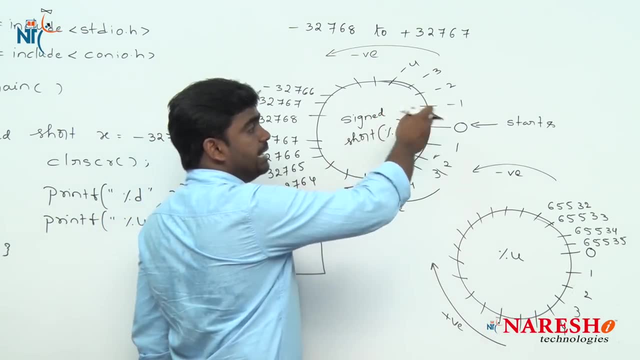 that is why compare these two, Just compare These two circles. almost same, But this is completely positive. Just this is divided into positive and negative. But exactly how many circles are there? How many circles are there? How many circles are there? How many? 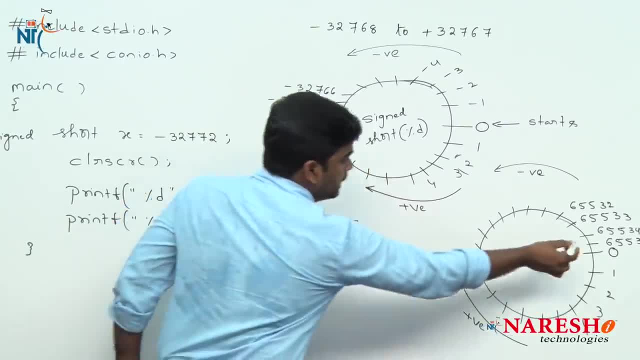 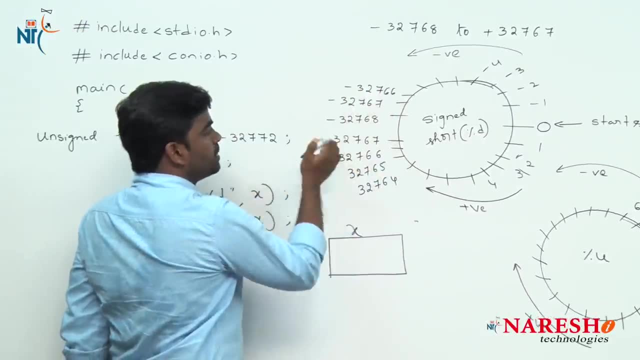 numbers in both the circles are same, So while counting, So this counting and this counting, almost same. Minus 1, minus 2, minus 3, minus 4, and so on. keep on counting. Minus 32768, minus. 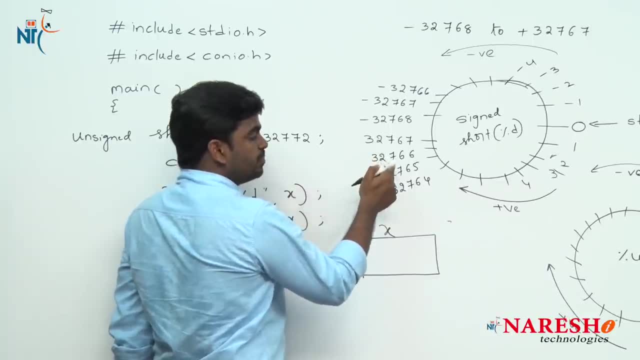 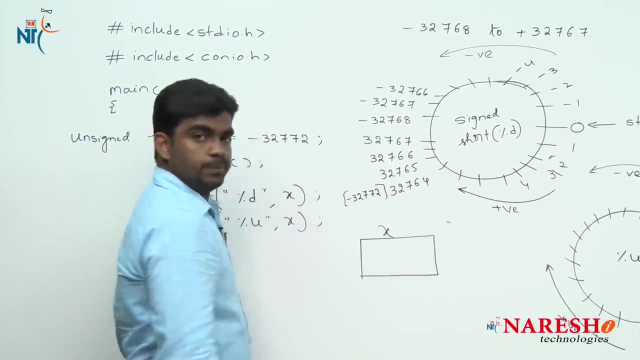 32769, minus 32770, minus 32771, and this is minus 32772.. Minus 32772 is equals to 32764.. Here it is. So this is minus 32772. So this is minus 32772. So this is minus 32772. So this is. 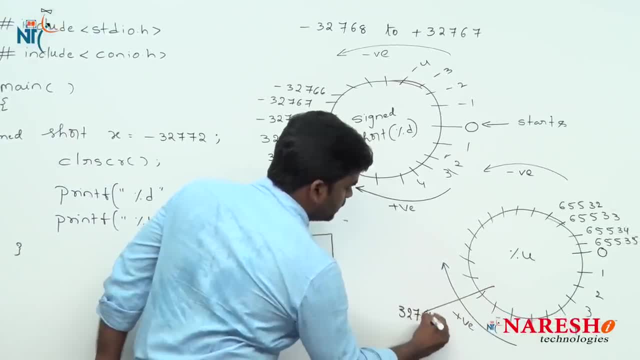 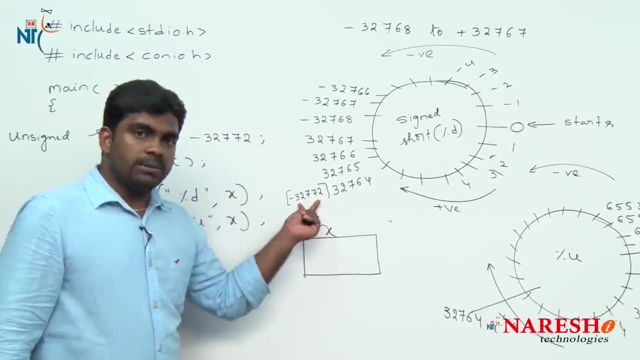 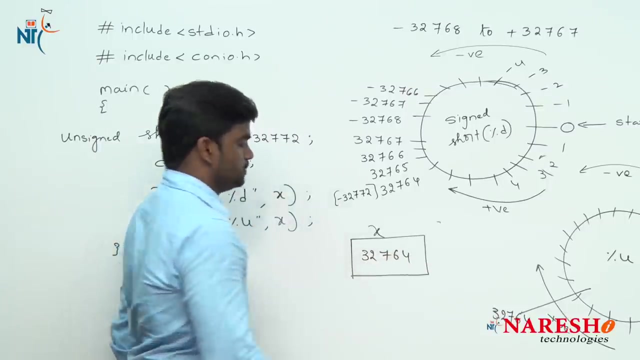 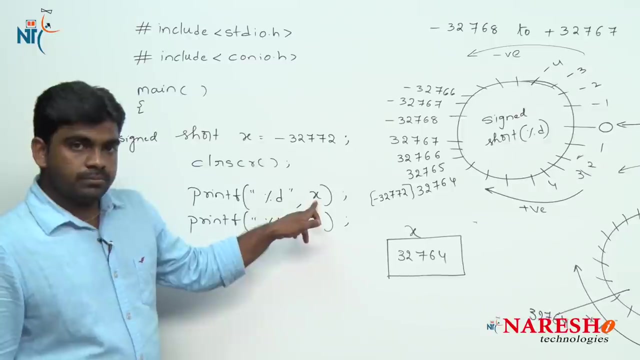 somewhere 32764 will be present in this circle also. Both circles almost same, So here it is minus 32772.. In place of that, what value will go and store? 32764 will go and store. 32764 will go and store. Now we are printing the text value, So as usual. 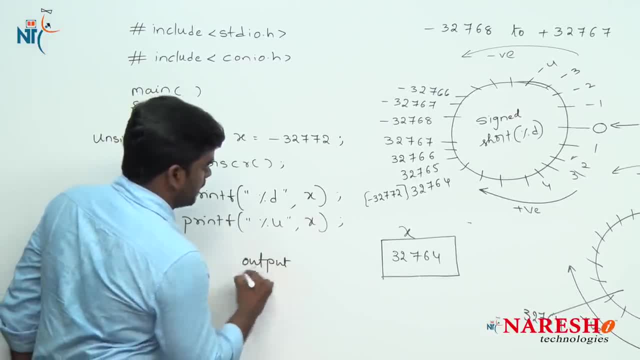 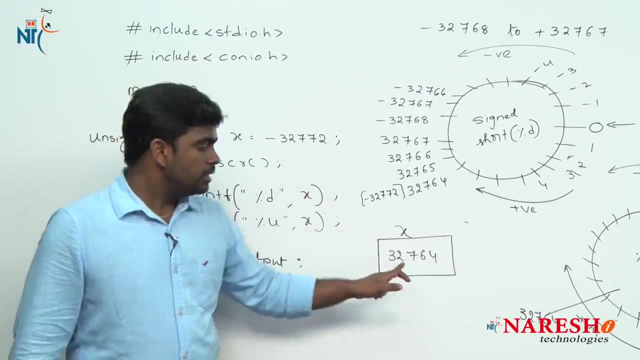 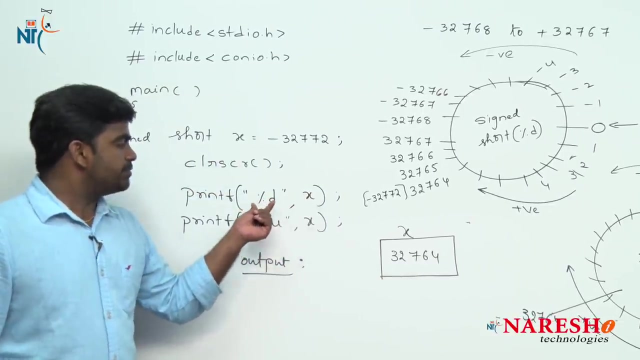 it will collect the text value. This is output. It will collect the text value. What is the text value? 32764, not 32772.. What is the value? 32764, it will collect After collecting 32764,. what format specifier you have given is also important. What is the? 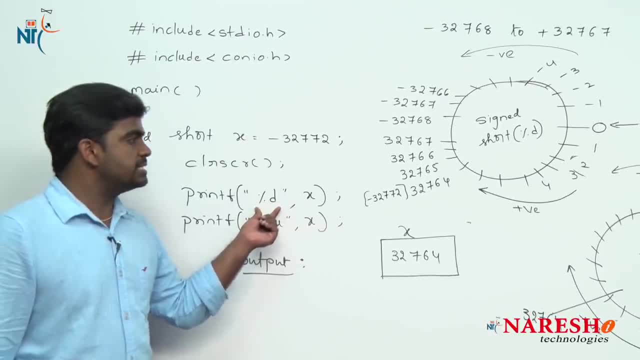 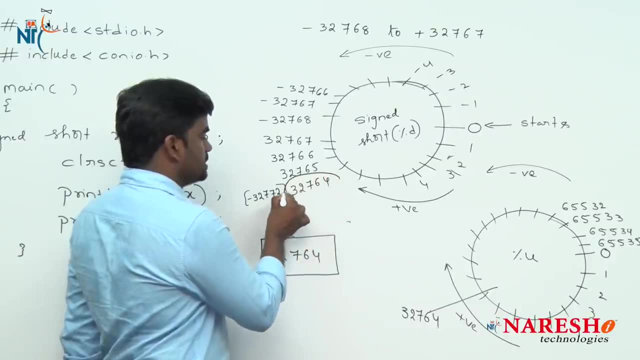 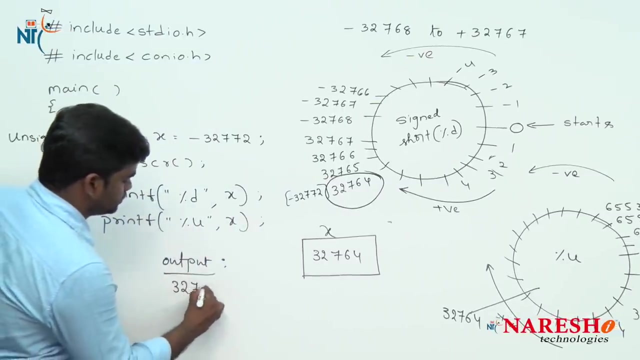 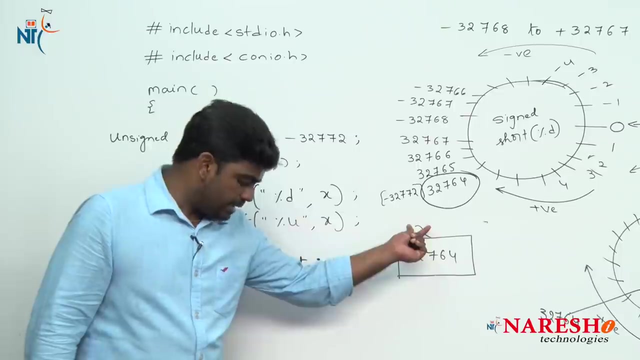 format specifier: %d. %d means what. This is the circle. In this circle, 32764 is present or not. Yes, 32764 is present, So it will print: убительно 32764, only 32764.. Next, again, x wished for collecting What is the text value. 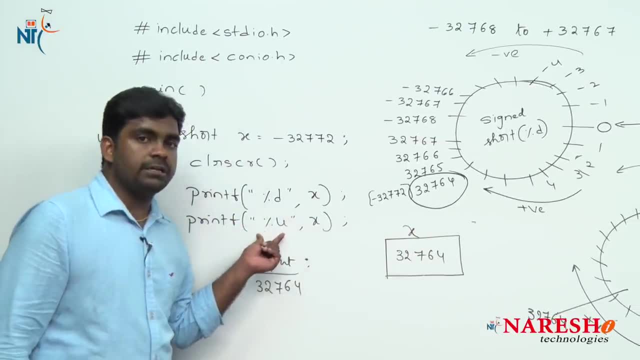 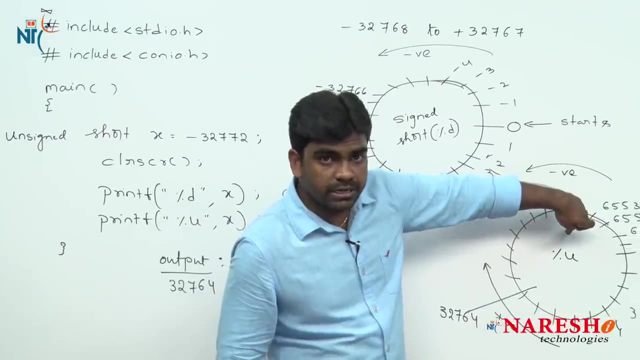 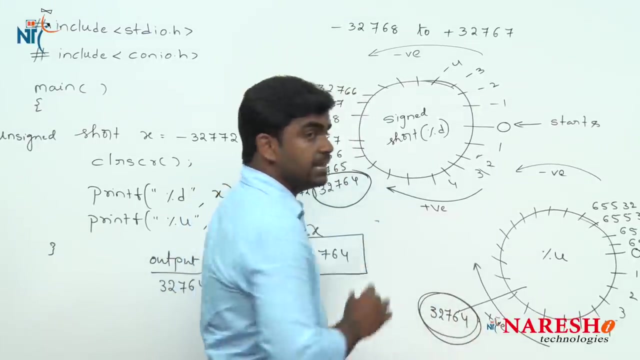 32764.. But what format specifier you have given? %u is a format specifier. See here, %u is a format specifier. In this format specifier 32764 is present or not? Yes, here it is there. So it will be this way. So if the if we look at the nation of Britain, then we have 32764,. 22764.. Here, 32764 is there, So there are 1,, 2,, 2,, 3,, 3,, 4,. can it be 18 birds, 3 birds, 2 birds, 2 birds. So 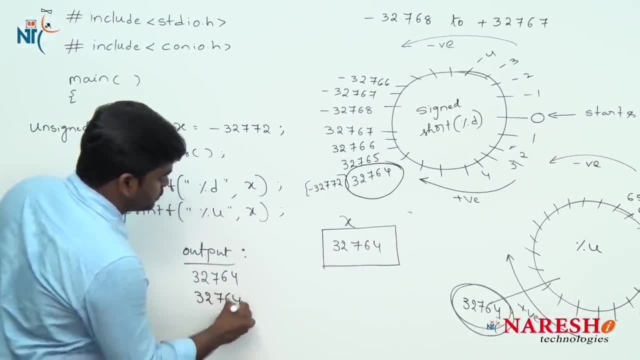 must come on. the only list of red dost, 3 more 3 birds is there. So last, then next number of birds will print the value once again, 32764. it is printing, So any relation between input and